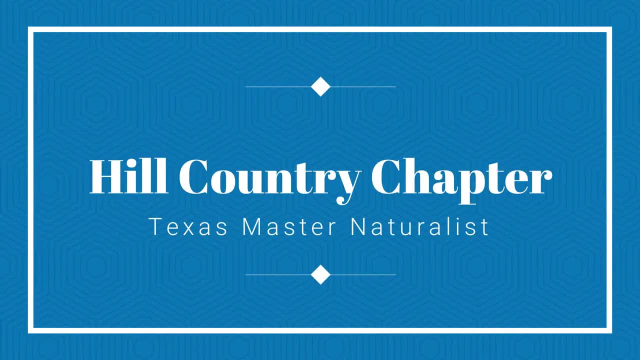 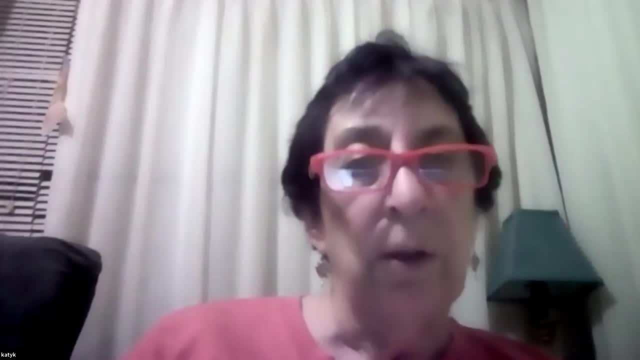 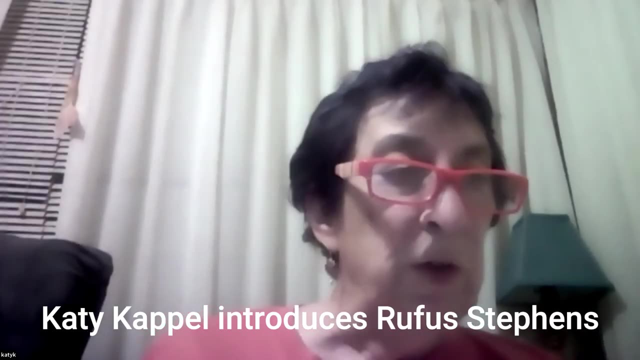 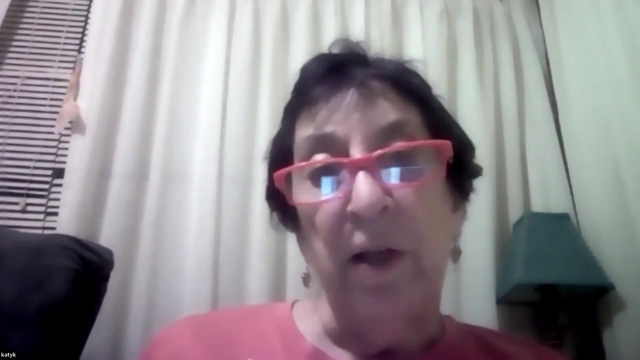 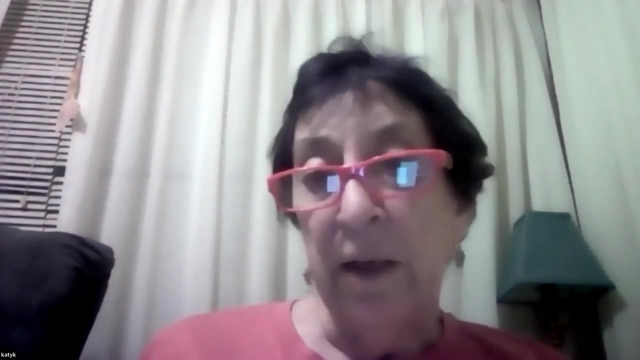 There you go. Okay, well, you new students have already had a chance to meet Rufus Stevens, but for those of you that have been in the closet for the last five years, Rufus is a superhero of the master naturalist. He is one of the people that thought up the idea more than 20 years ago. 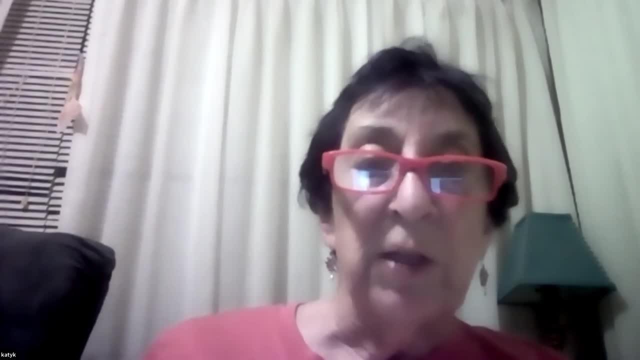 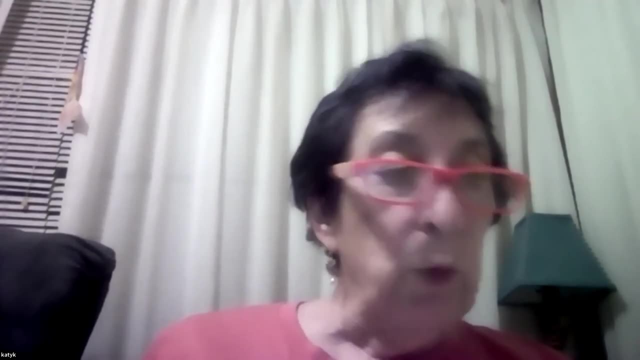 and he's been working as a wildlife biologist ever since. He spent some time in Kansas doing this kind of work and then was 23 years with the Texas Parks and Wildlife Department, so he knows what he's talking about. He has written a book with Jan Reed on attracting birds in the Texas. 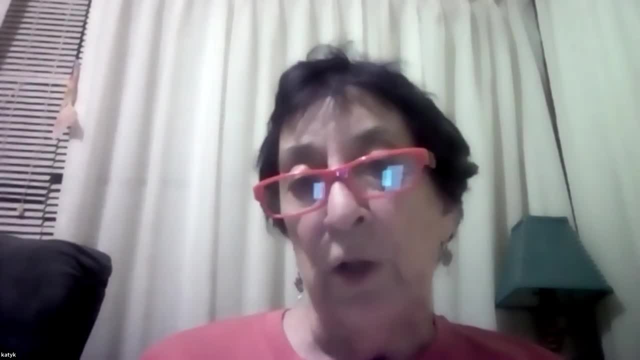 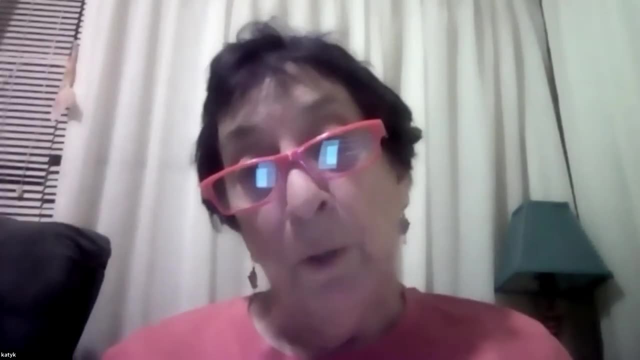 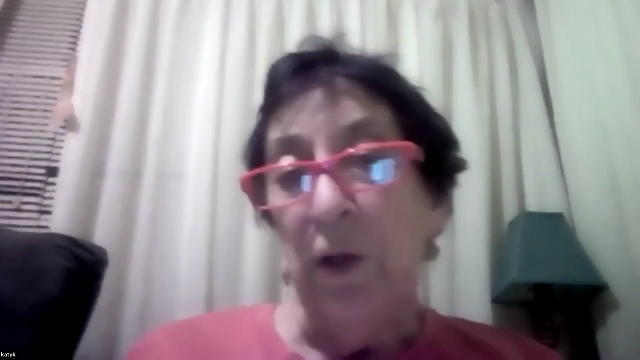 Hill Country and I know we have that at the Riverside Nature Center, but if you have trouble finding it, it comes from the A&M Bookstore, which is a good place to find any books you need. So I am excited to hear him explain something that everybody that's new to Texas wonders. 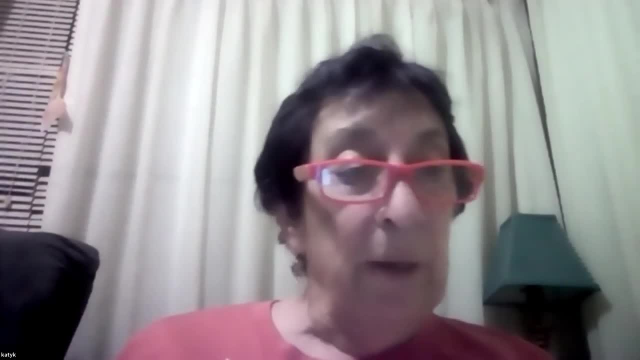 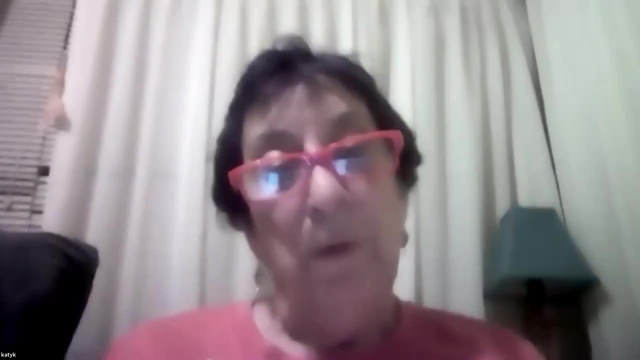 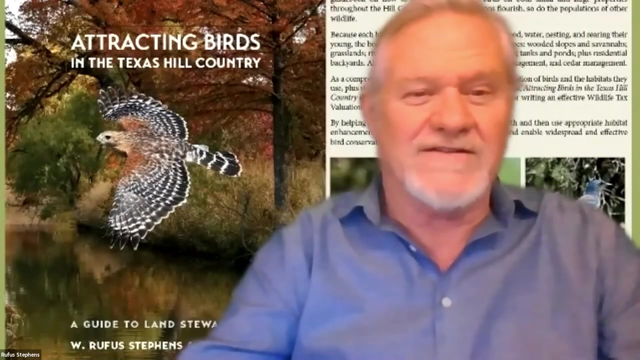 If you have moved here from somewhere else, I'm sure it has entered your mind. why in the world are there so many deer walking around? So, Rufus, it's all up to you, All right. Thank you, Actually, it's also great to see. 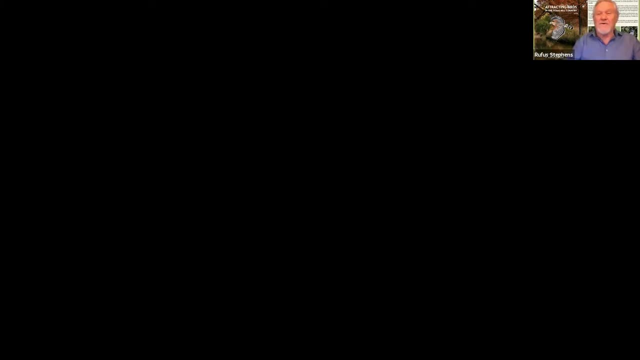 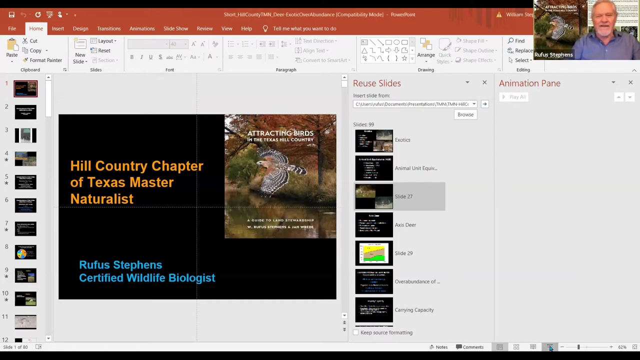 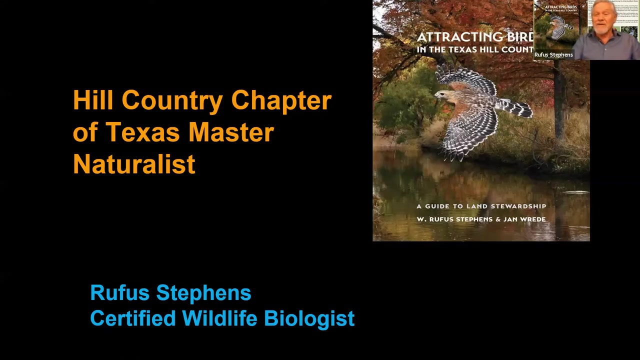 or to recognize that a whole bunch of friends are on there: Lucy and Andy and Nash and Coey and Louisa- just a bunch of folks that I know, And I'm sure there's other folks that I missed. So what I'm going to do is this is: 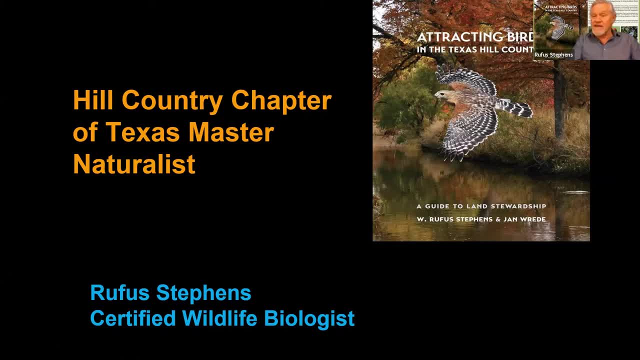 actually a presentation that I normally give to the class. Some of y'all may recognize this. We're going to try to go through it pretty quick. I'm going to just kind of hit some of the highlights and try to give us enough time to have a discussion. 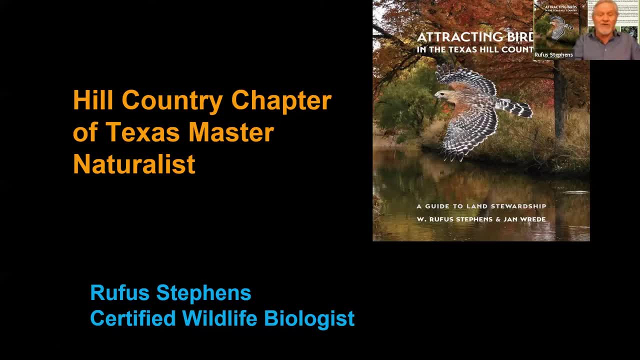 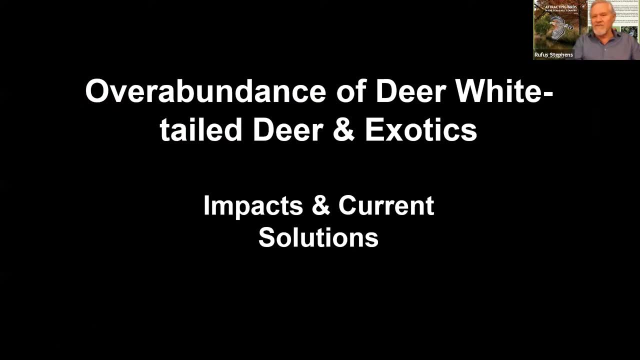 at the end- And this usually topic usually brings up lots of questions- And what I'm going to talk about is the overabundance of white-tailed deer and exotics. Basically, I'm going to talk about the impact and current solutions, And that's kind of. 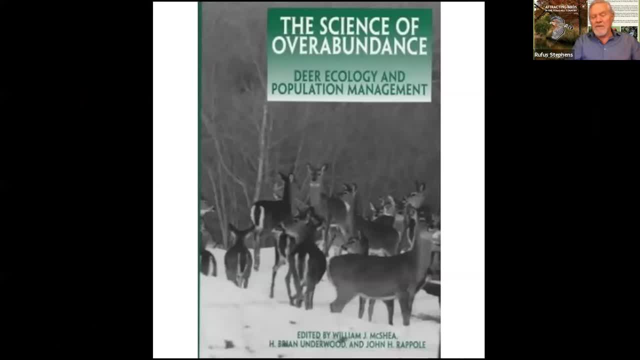 where we're going to really get into our discussion. This is a topic that actually they have written books on And I'm going to talk a little bit about the impact and current solutions. So it's been thought about and discussed a lot And we certainly have our share of issues related to. 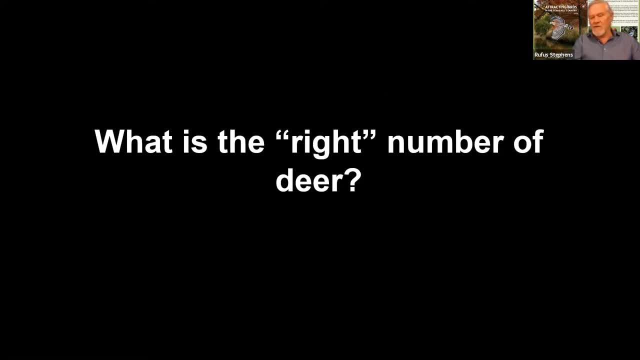 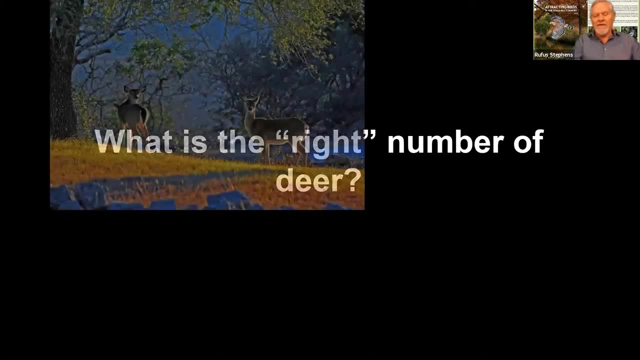 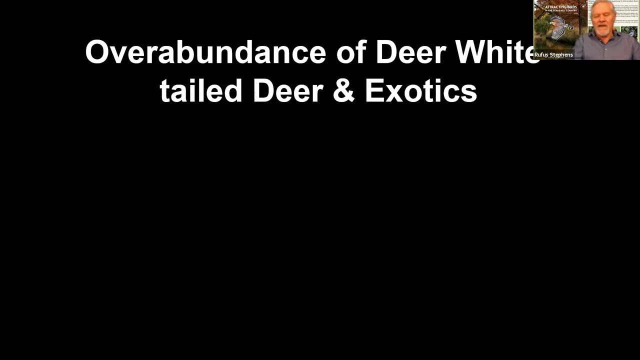 overabundance of deer. So we might start with what's the right number of deer, And we're going to talk a little bit about that as we kind of move on. And so what is the right number of deer out there? And I'm going to just touch on white-tailed deer biology and exotic biology very quickly. 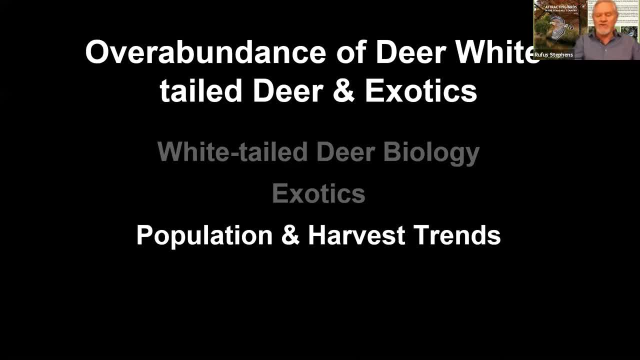 We're going to talk a little bit about population trends and harvest trends, And then we're going to talk a little bit about ecological impacts And we're going to finish with talking about population control options. And that's usually, but there are other aspects. 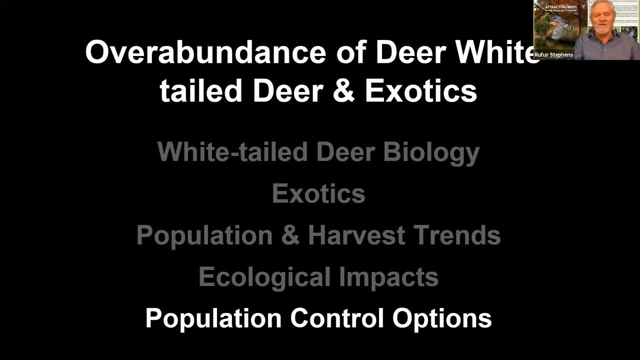 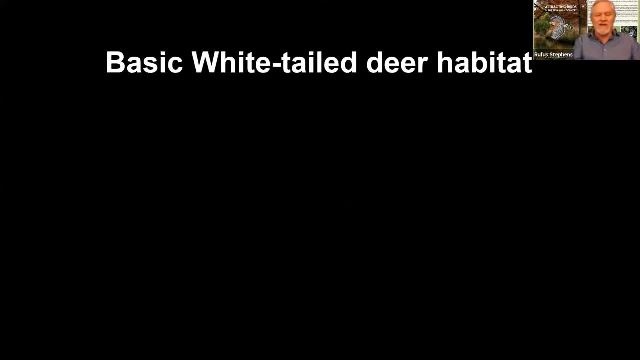 of this that people will have questions about, But that's usually the right number of deer. That's definitely a important issue. So white-tailed deer, biology and exotics And so kind of the basics of food for white-tailed deer: they basically eat forbs and browse, which are woody plants. 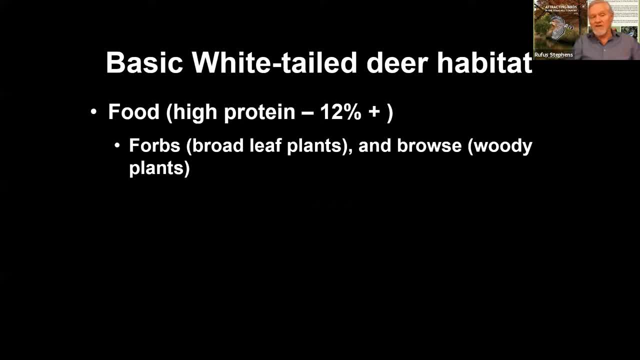 And the protein content in those food sources is greater than 12% protein And at times their biological needs- like a nursing doe, that's over, that's as high as 20%. So and they also have a requirement, those basic components of habitat, food, water and cover. 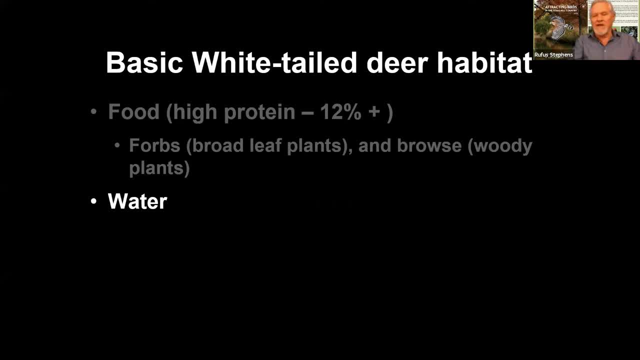 water, typically within a mile, And so there's really not many places in the hill country that we don't have water within that amount of time, amount of space. And so you know we're going to talk a little bit about population control And I'm going to 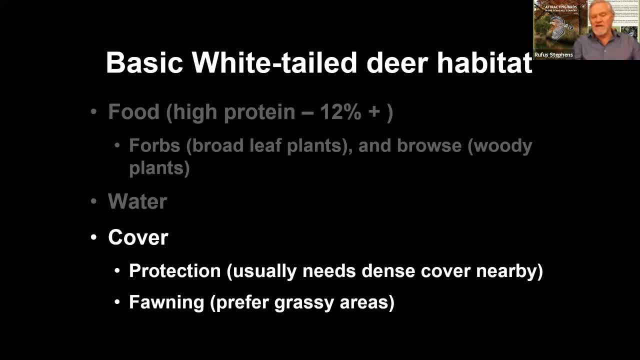 also cover. The basic types of cover is basically protection And that's dense cover nearby And usually that's within 100 yards, is kind of their basic requirement. If it's further than that and someplace they're wanting to feed like an oat field, they'll do it at night or when it's. 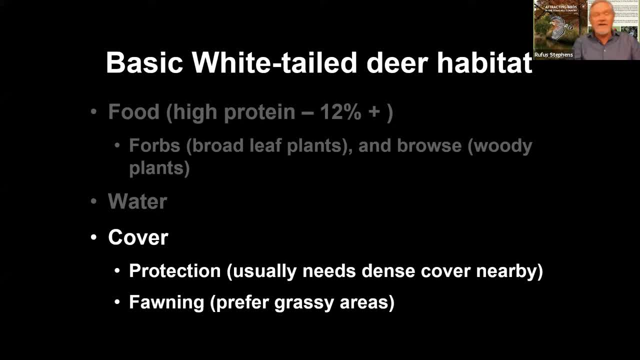 or in the evening, And actually deer are copuscular. There's a $10 word for you: copuscular. So they're not diurnal, They're not nocturnal, They're copuscular. That means that they are active. 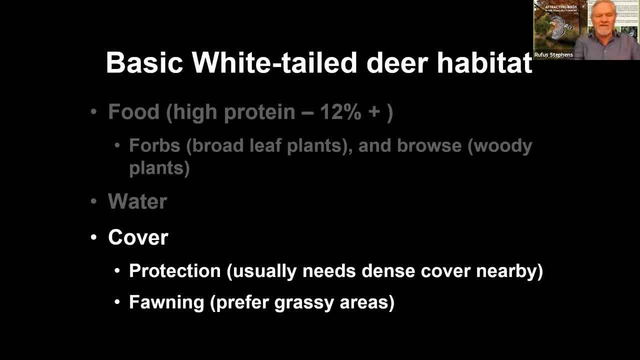 in the morning, in the evening, Those are their primary active activity periods. So the other aspect of cover is fawning And basically those are grassy areas to hide their fawns And they, for up to two weeks they will not. they will nurse their fawns and then leave them And don't. 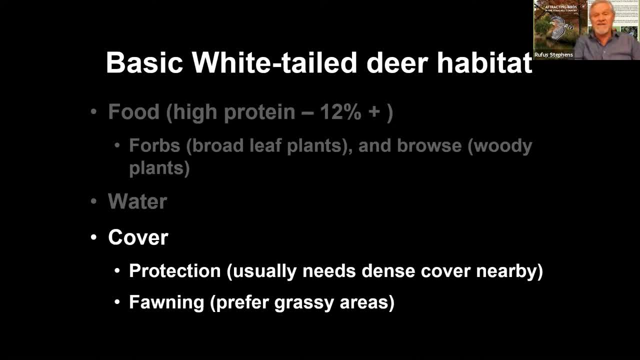 come back. They're not going to come back. They're not going to come back. They're not going to come back until they nurse them again, And that can be several hours, And people often think they're abandoned, and they're not. That's a common issue, right? When you know, in June we all of a 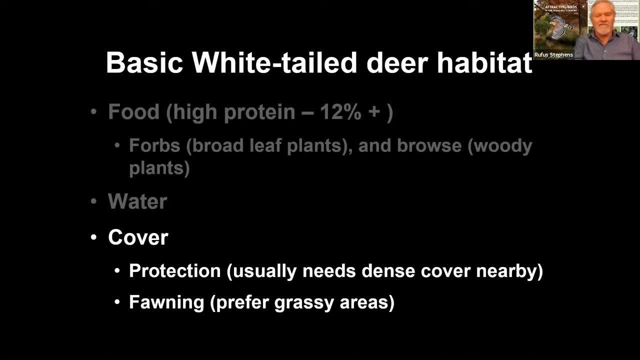 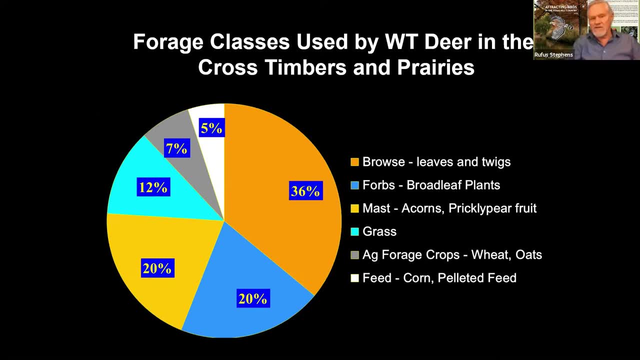 sudden Parks and Wildlife gets lots of calls about abandoned fawns And it's like, no, they're not abandoned, They're food. The basic thing here is to remember that. browse the leaves, twigs of woody plants, forbs, broadleaf flowering plants, you know some people call them weeds. 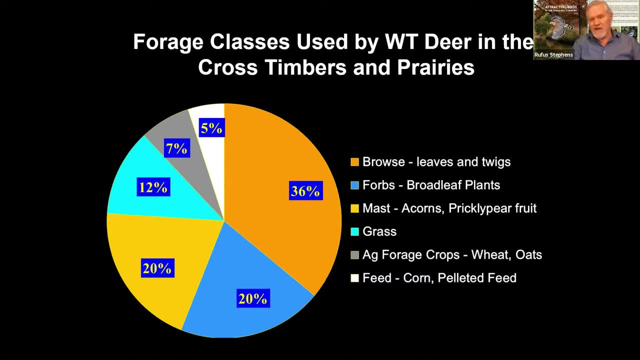 some people call them wildflowers- and mass, which are acorns and nuts, and includes things like prickly pear fruit. That's 75 plus percent of their diet. Grasses make up very little and it's a very specific, very specific timeframes that it does, when it's much higher protein. 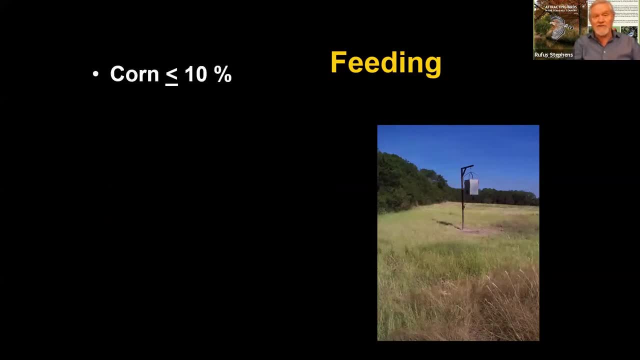 Feeding. This always comes up, And so we got to address it. Understand that corn is less than 10 percent protein, And remember I said that they need at least 12 percent in their diet. So some professors, folks at A&M, will call it beer for deer, And so it's a high carbohydrate but low. 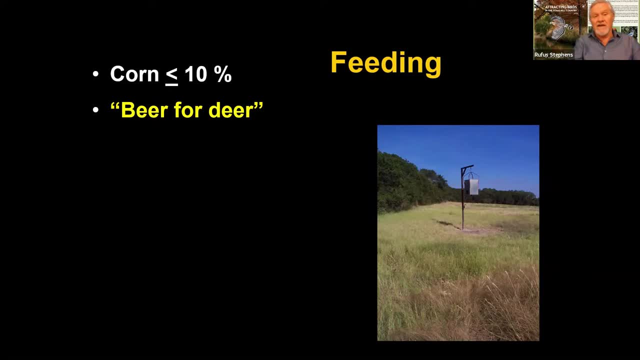 protein diet And it is. it's like I would like to think that I could live off of that, But I know I probably couldn't just drink beer and survive Again. protein, high protein. they need high protein more greater than 12 percent. The other problem with now we're going to get into: 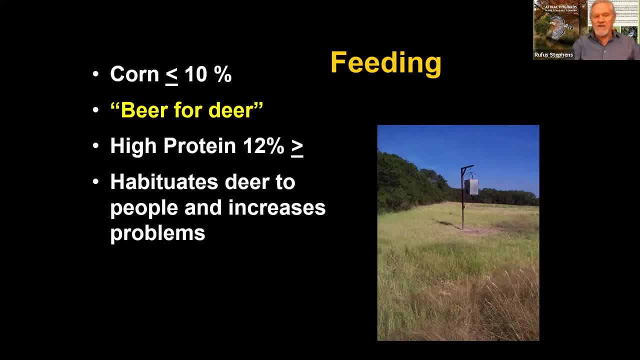 just what are the problems associated just with feeding? So one of the things that habituates deer to people and increases problems with people. One of the things is it also causes a lot of problems with people. So one of the things that habituates deer to people. 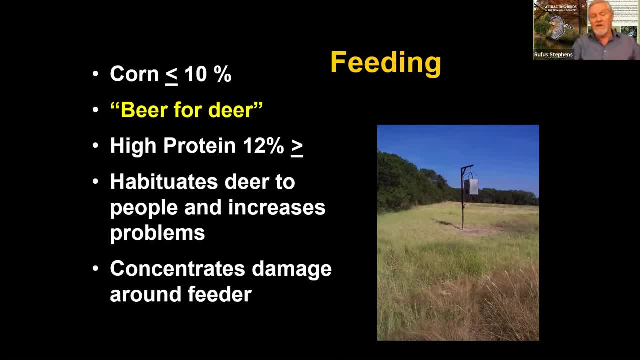 is, it concentrates damage around the feeder. And when there's a regular food source that shows up at a certain time, whether that's by a feeder or by putting it out, deer will not travel as far. There have been studies that have shown that they will not travel as far within the. you know. 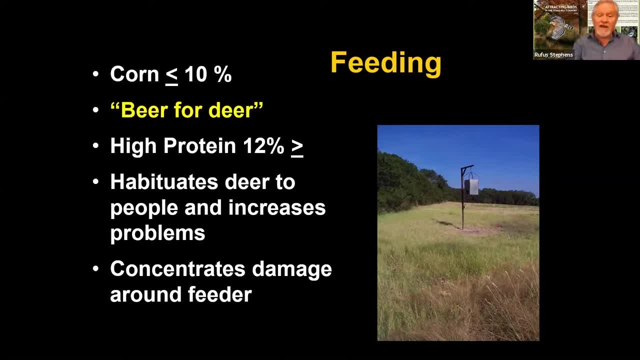 Pavlov's dog within the back of their mind. they have that feeder going off, And so they'll go and, and so that that means that around the feeders they tend to overutilize the habitat where, if those feeders were not there, they would not. they would be more evenly distributed across the 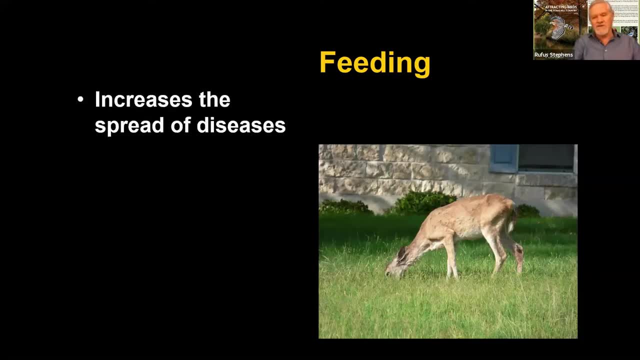 landscape. It also increases disease problems and the spread of diseases. And this is looking at this deer that's in a yard. This is in Garden Ridge, near down the outskirts of San Antonio. this deer, not only can you tell from its coat but its hip bones. this is a deer that's in really. 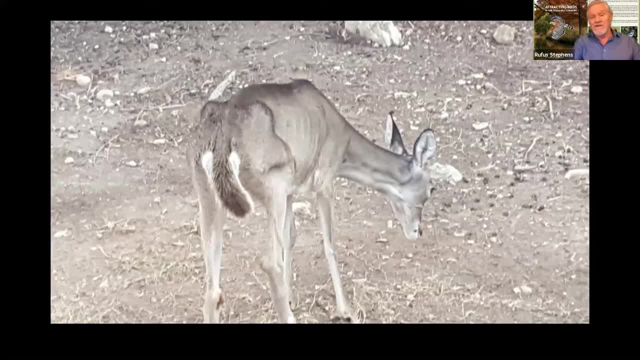 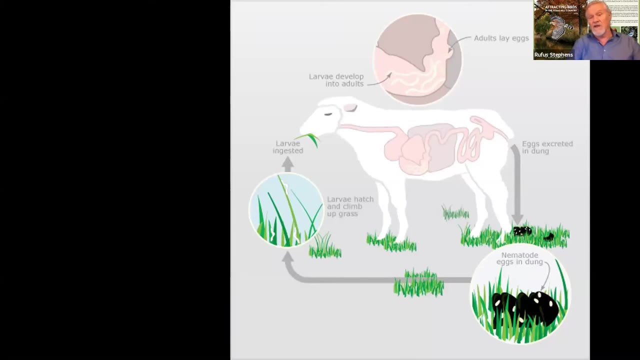 bad shape And this is an extreme- a deer in extremely bad shape- And the reason for this? for both of those situations, the most common thing that we see is these are high parasite loads And what we with with Parks and Wildlife. when I was with Parks and Wildlife, we did some work on looking at what was 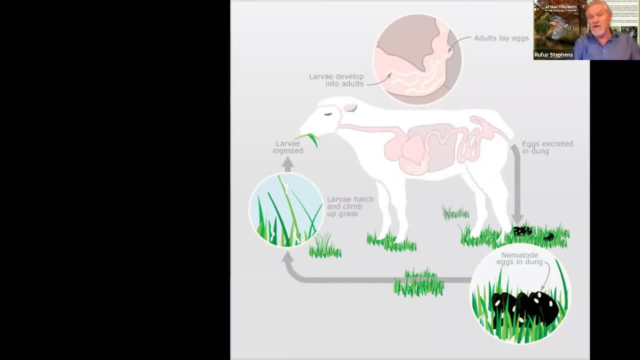 the parasite load on some of these urban deer And they were dramatically magnitude higher than deer in in normal areas or in rural settings. So what they the? the problem becomes is you're concentrating animals that potentially are, you know, expelling eggs from, from parasites, And then they're eating close to the ground, They pick up. 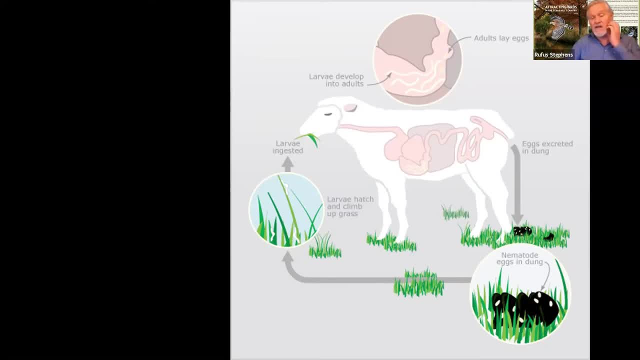 those parasites And these some of those disturbing photos that I showed of deer. we often get people going: oh, this has got to be some kind of CWD, chronic wasting disease- which we do have in Texas, but it's. 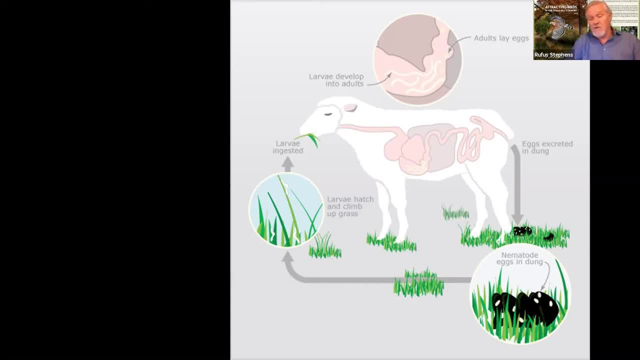 not in really any of our urban areas and and or or or cities or communities other than Del Rio. It is in the Del Rio area now, but is that these are almost always parasite problems? When we look at those deer they have, they have typically three things: high parasite loads. 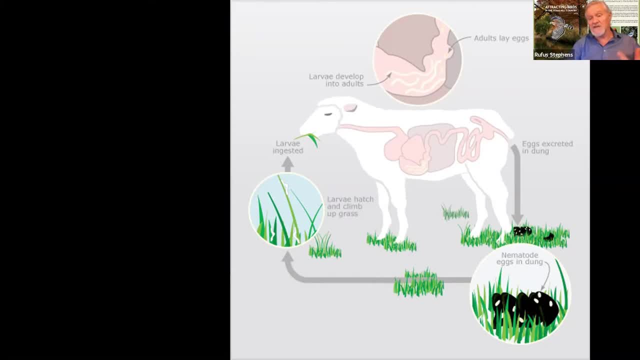 very high parasite loads. They'll have acidosis, which I'll get into in just a second, And and and they'll have, they'll have, they'll have a lot of parasites, but they'll have. they're not, they're not, they're not really, they're not, they're not really, they're not really. 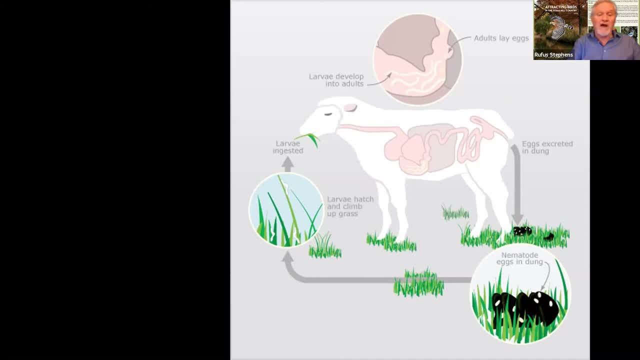 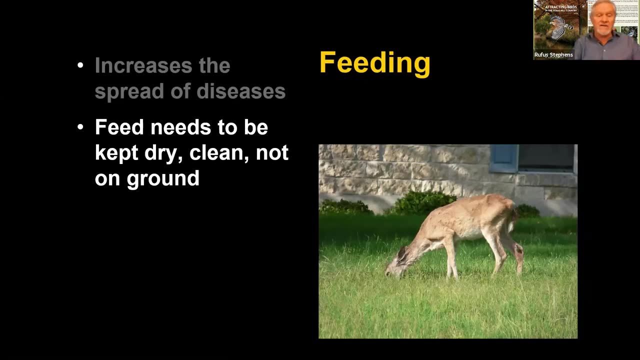 aflatoxin, which will all be part of the problem with uh feeding deer. so if you feed, then you know. the thing is is to keep it dry clean, not on the ground. um. acidosis already mentioned. acidosis is basically an acidification of the rumen, um and or the or the bloodstream. it's basically from 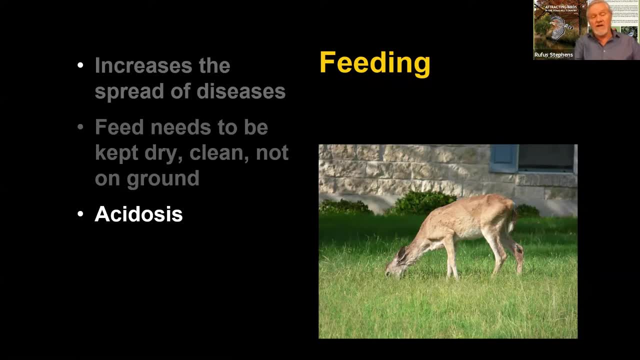 getting too many carbohydrates and you get acidosis. uh, which is common in urban deer. um, aflatoxin, which everybody should know that if you look at a bag of corn, flip it over, it's it'll be on. usually on the back side be a little. statement says less than 20 parts per billion aflatoxin. 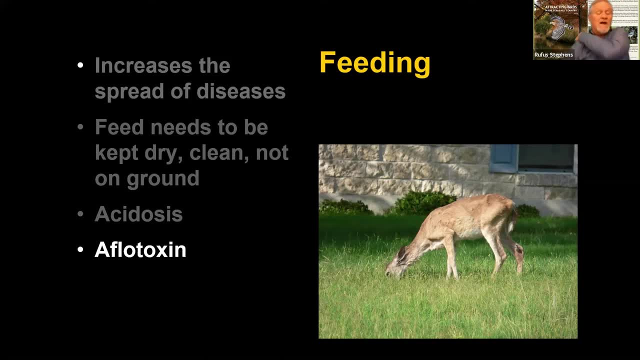 some says less than 50 parts per billion uh and aflatoxin at 200 parts per billion can be detrimental to deer uh. the problem is is, even though it has those statements on there, uh aflatoxin can be varies dramatically in uh. agri-life did a research a number of years ago. 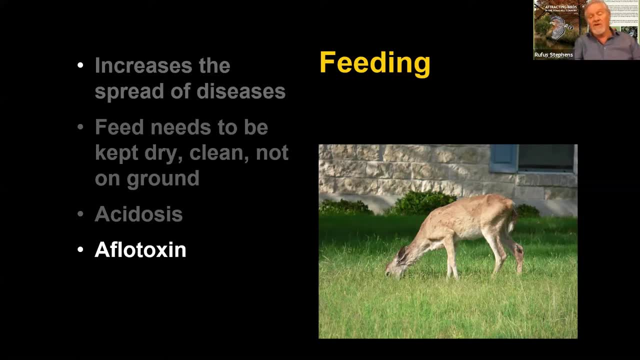 and basically found that, um, there were considerable uh uh bags of corn that would have uh 500 to a thousand parts per billion. uh, so enough to impact deer's uh health. um, the bottom line is is: you know, if you care about the, about healthy deer, don't feed them. 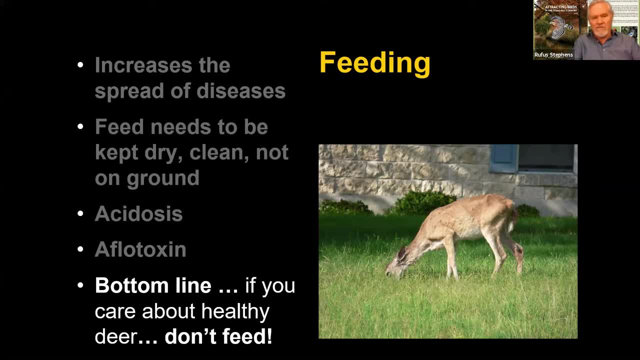 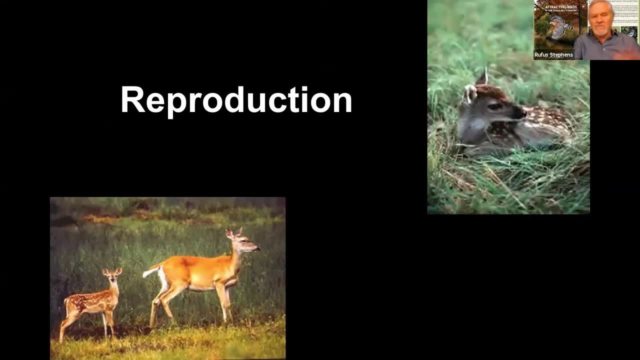 uh, it's just not good all the way around, even if you go. well, i'm gonna feed them higher protein. no, it just causes problems reproduction. um, it's important to know that that with uh, twins are normal. actually, singles are almost as common in a healthy deer as are triplets, and so occasionally, 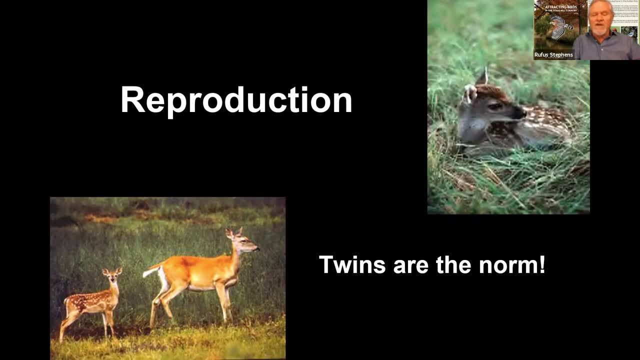 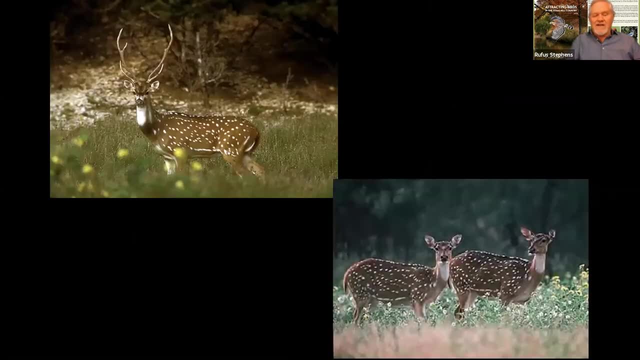 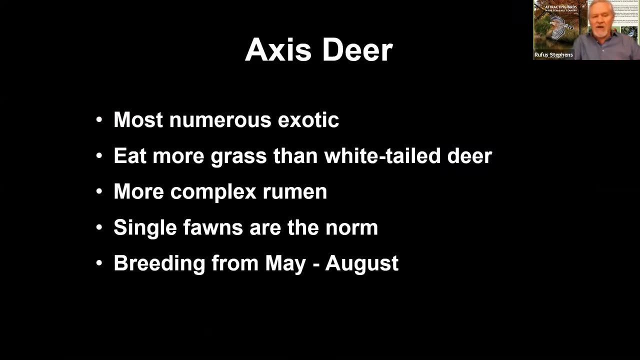 we'll see triplets and people will talk about triplets. um, uh, twins are normal, so, uh, do a little bit. talk about the exotics. uh, the main exotic that we're talking about is, uh, axis. deer and axis are probably the most numerous. um, they more grass and whitetail deer. 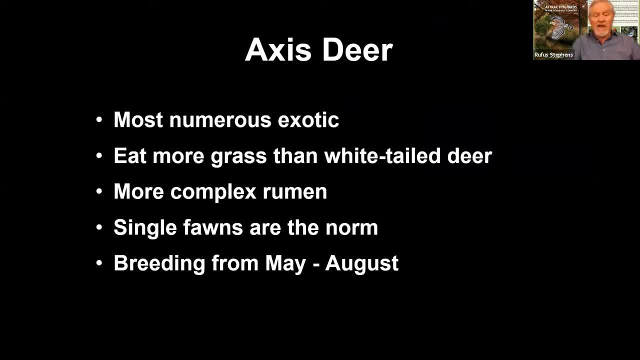 that's because they have a more complex rumen um and digestive system, and so they can. they can- they can eat more grass and whitetail deer, and so they can. they can eat more grass and whitetail deer, eat a lower quality, lower uh uh quality forage and and still do well, single fawns are the norm. 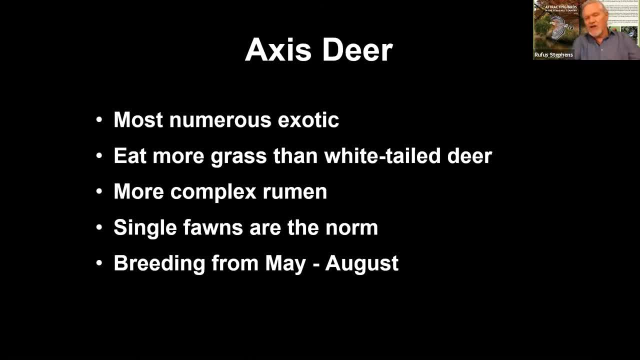 uh, breeding is typically from may through august. uh, and it is tends to be because they come from uh, india, uh, they are tied to, just really biologically wired, to a rainy season and in in india, it's only one time they have one rainy season, uh, the monsoon season, and that triggers 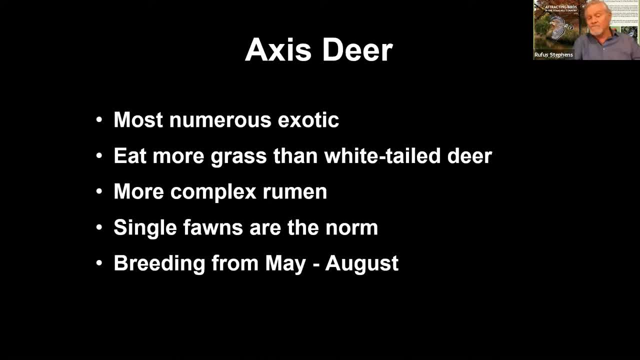 their, their cycling and um. but in texas we have two rainy seasons, we have may and june, and basically september and august or september and october, and so we can get access almost fawns almost any time of the year, and and so people may have seen fawns fairly small, uh young. 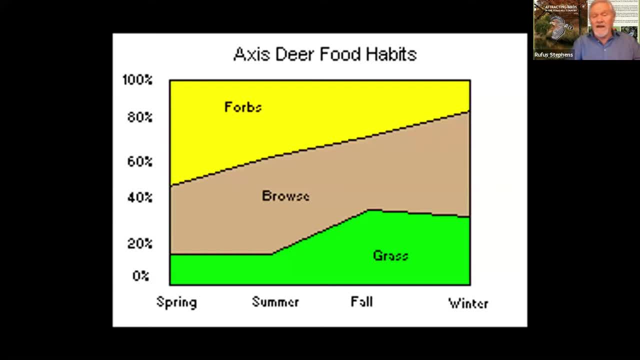 fawns in the wintertime. uh, one thing about their diet. it again: they they'll eat more grass, uh, and can eat, eat, uh, low quality forage food, but they prefer the same things as whitetail deer. so, and from a competition standpoint, they eat, they'll eat, forbs and browse, which is the same. 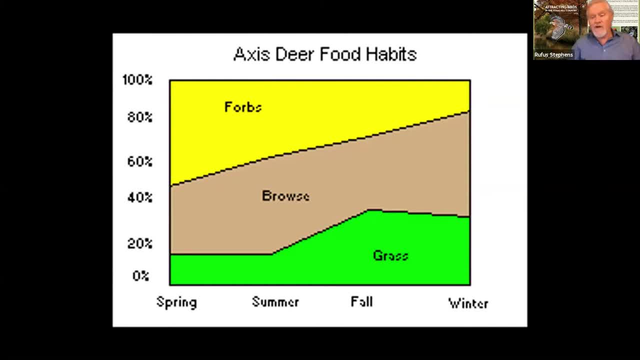 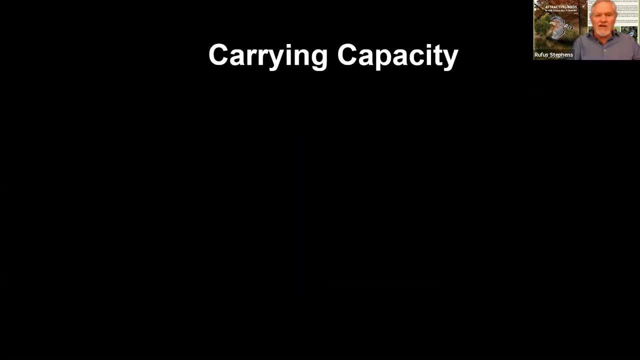 thing: whitetail deer eat, but then they can shift their diet to grass if they need to. whitetail deer cannot do that. um, a little bit about population. um, one of the things is carrying capacity. when we're talking about populations and their levels, uh, carrying capacity, important concept. 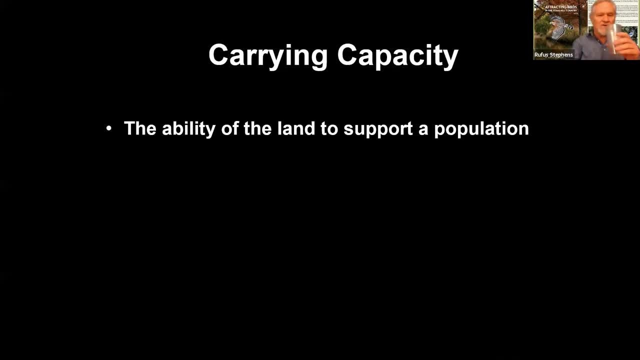 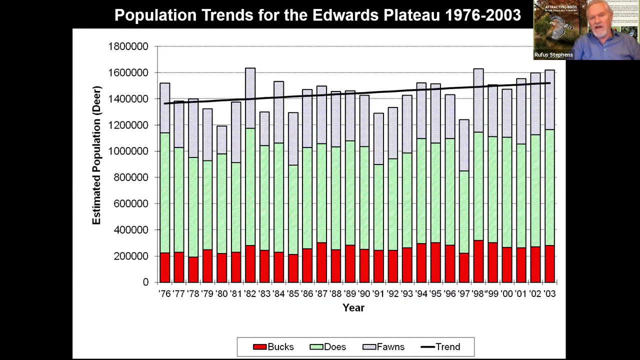 it's basically the ability to land to support a population of wildlife and basically reproduction decreases as the population approaches carrying capacity and as the population exceeds carrying cap uh carrying capacity. it's basically the ability to land to support a population of wildlife with a single uh uh. 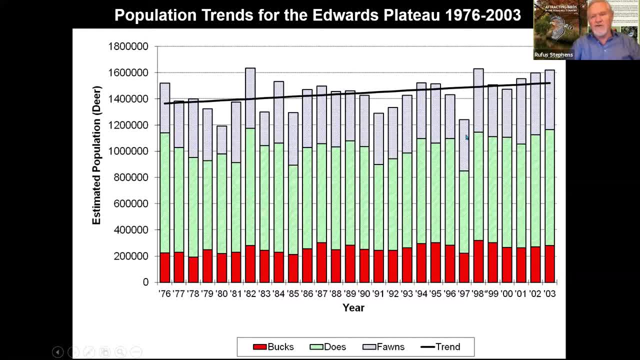 uh, uh, uh, look at this and see that there are less than one fawn to every doe. So twins are normal and you know we're seeing times where there is maybe only one fawn to every five does. So, uh, that's that increased mortality in the fawns, uh, associated with, um, uh with, with exceeding 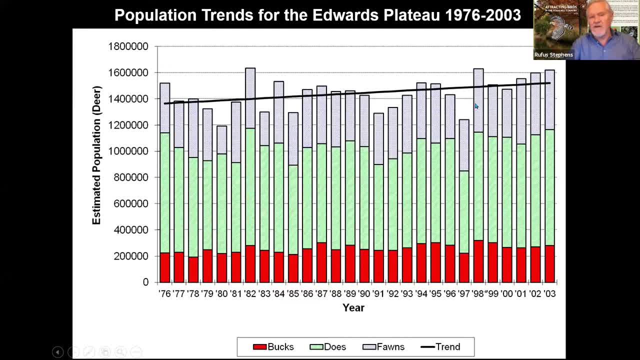 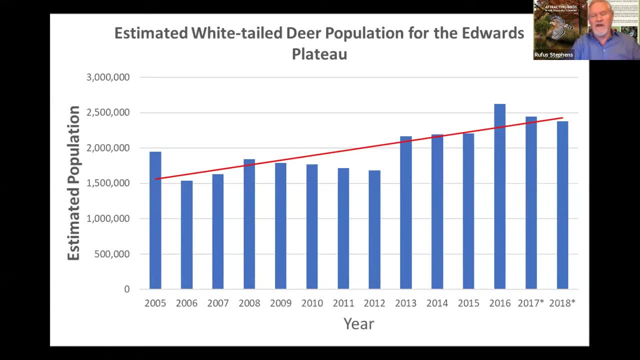 carrying capacity. And so we in Texas, we in the hill country, we have been exceeding carrying capacity for white-tailed deer um ever since the 60s. Um the uh- this is just more recent data for the Edwards Blatch. So um, uh, the hill country, um, and uh, in 2005 they uh Parks and Wildlife changed the survey. 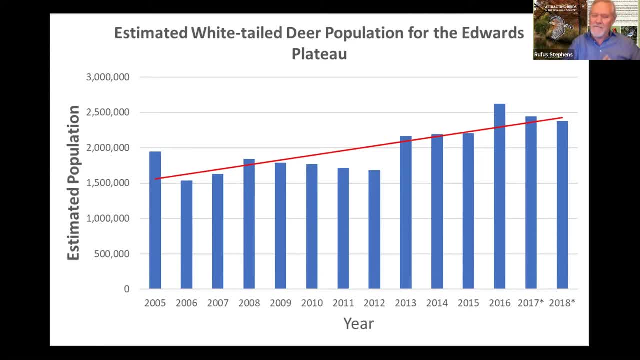 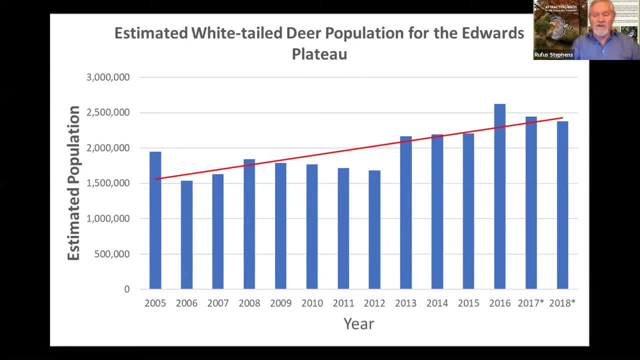 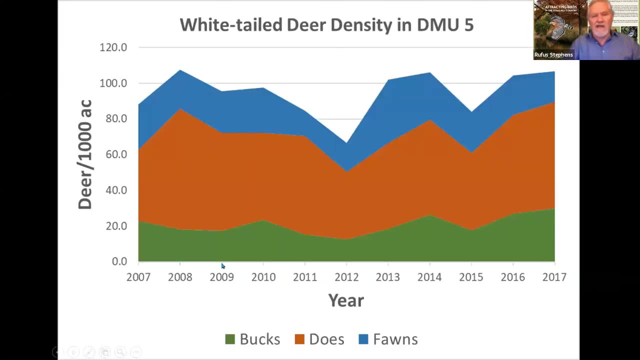 like an increase over, you know, the past, uh, 13 years, But that's probably in the long term. uh, there's, there's an increasing population, but it's oscillating. Again, it's exceeded carrying capacity. Here's just another way of looking at, uh, the trend over kind of that same time frame. 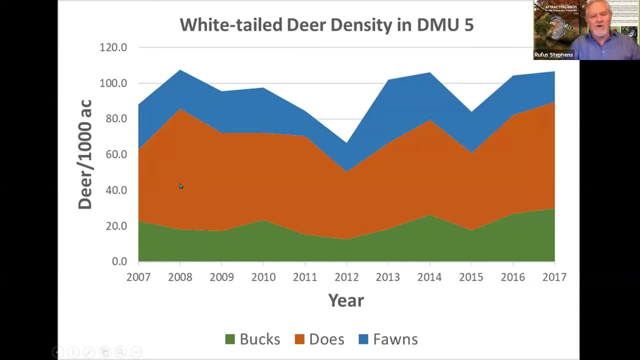 a 10-year period and basically looking at the number of does They're here in orange or red And the number of fawns in blue, And you can see that that's a uh, that there are significantly more uh does than fawns And that tells you that population's not in very good health. 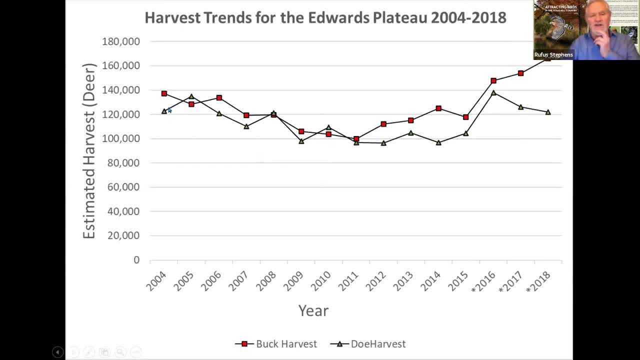 Um harvest, So how many deer are harvested? So uh, this, this number of uh uh. prior to like back in the 70s, when, when doe tags, when the harvest was allowed, That uh, the number of of um uh does that were harvested per buck were about uh, well before that. 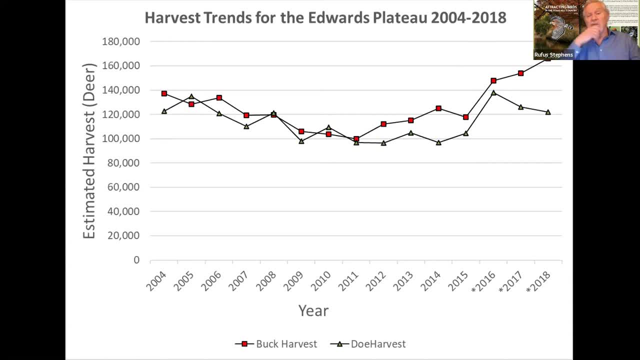 they weren't allowed. But once it started it was basically about half the number of does uh compared to bucks. It's gone up and then it's it's. it stayed pretty steady with an equal number And then it's just diverged a little bit in the past couple of years. 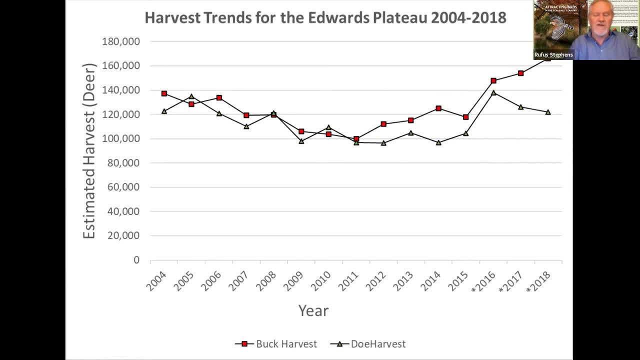 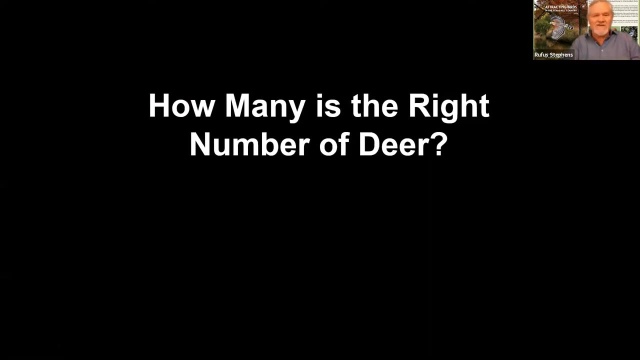 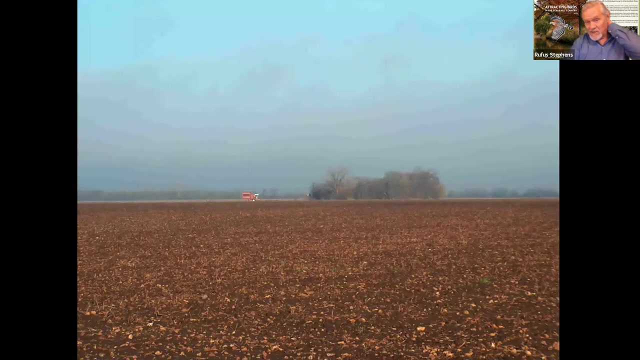 So there are more bucks harvested on average than than does, or just about equal in the long-term average. Um, but that's not gonna control the population. So how many is the right number of deer, as I asked earlier? Uh and uh uh. you know what is carrying capacity? Well, of a piece of property. So 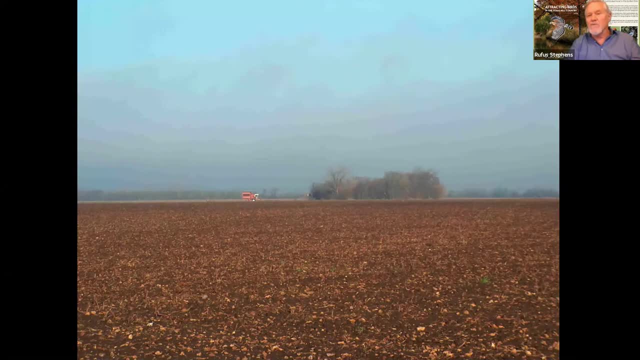 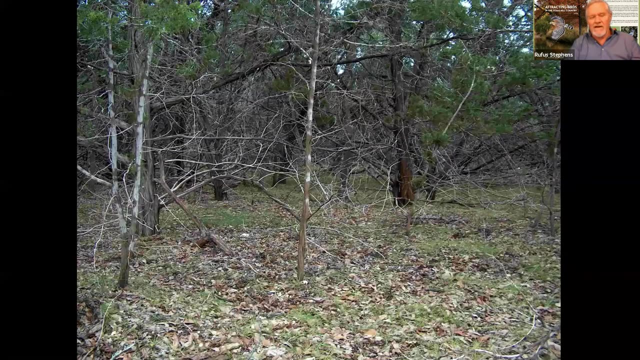 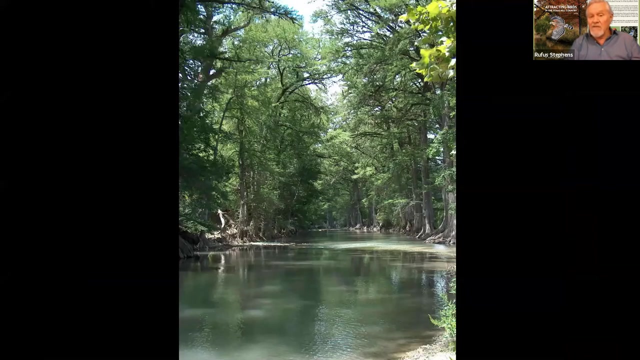 you know how many deer can live off this farm piece of ground? Well, until the crops are growing, not many, Uh. what about the cedar thicket? Uh, that doesn't have very high carrying capacity. This riparian uh habitat, on the other hand, may have some of the highest densities that we 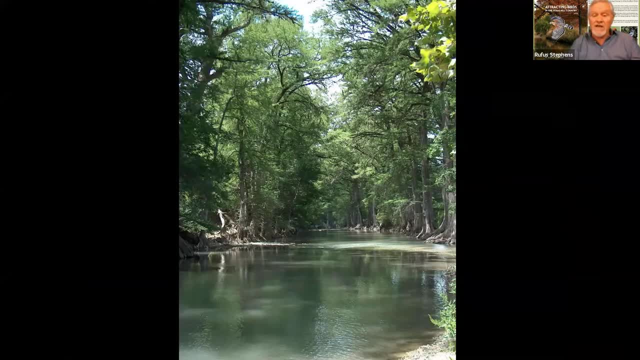 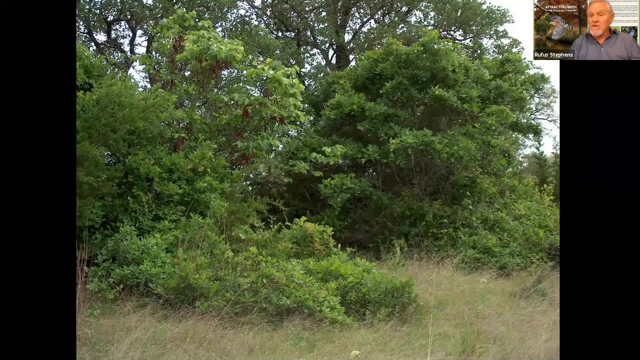 have in the hill country, Um, and or the highest carrying capacity in the hill country because of all the diversity that's there, Um, really good habitat from the Kerr Wildlife Division. And then just to add a little bit more information about the urban management area. 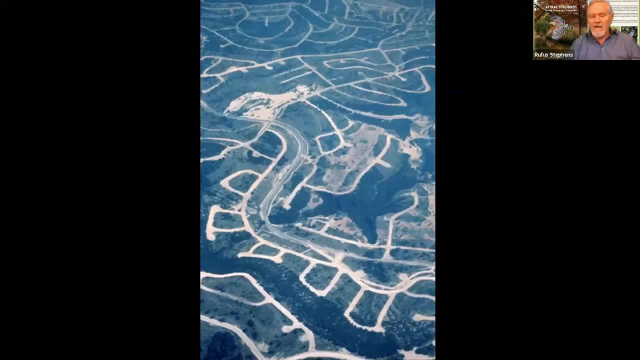 Uh, this has, uh, and even in uplands has, a good carrying capacity, And we often don't think about the carrying capacity in urban settings, but actually urban areas can have, um, uh, carrying capacities that are way in excess of the surrounding uh, uh, rural areas, Which is: 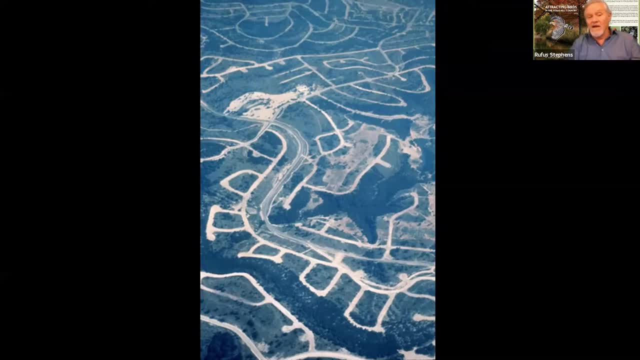 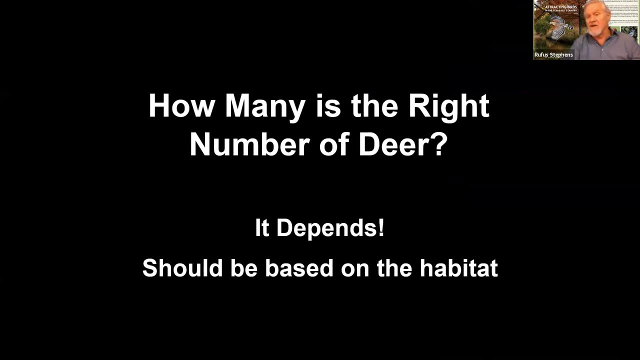 that biologists really didn't think would happen. um, so again, how many is the right number of deer? well, it depends, uh, and it's based on the, the amount, on that, on the type of habitat and the quality of that habitat. so if, if it's cedar they get, you can't have very many deer supported by. 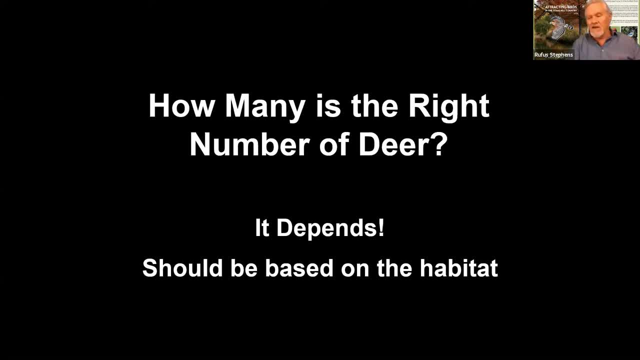 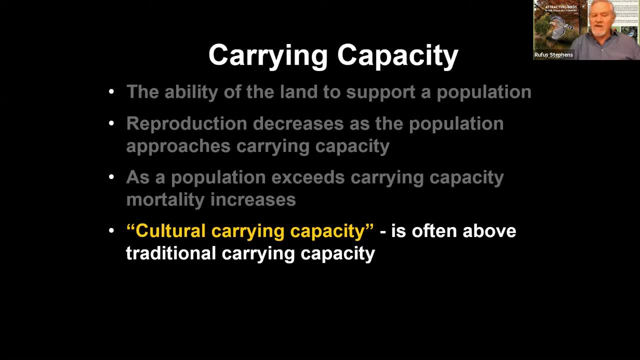 that, uh, if it's high quality, uh uh habitat, like out at the kerr area, well, you can carry more deer. then, um, one of the things about carrying capacity. we biologists often talk about cultural carrying capacity, and this is, you know, it's what, what will people tolerate? and it's often far above. 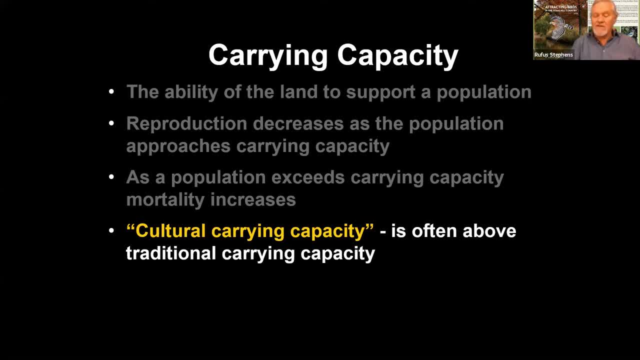 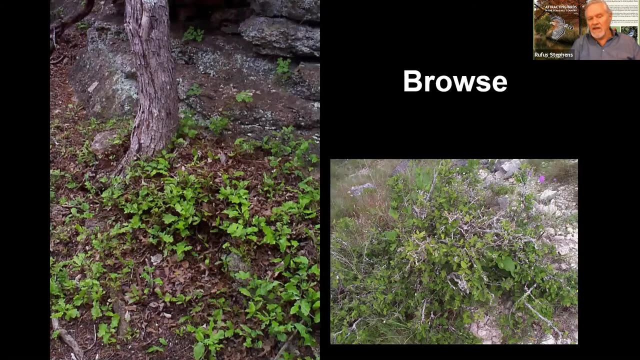 traditional carrying capacity. so we will tolerate a very high deer population, even one that is, uh, a detriment to the deer themselves. so what about the ecological impact? as I mentioned, den� برين deer browsers: They browse woody plants and forbs And we actually have plants. This is chinook here on the left and a cedar elm right here on the right. This one, this cedar elm, is kind of bonsai. It's very. it's probably should be about 10 feet tall. It's probably less than a foot. Chinook will want to do lots of resprouts and this and actually form like a thicket. The. 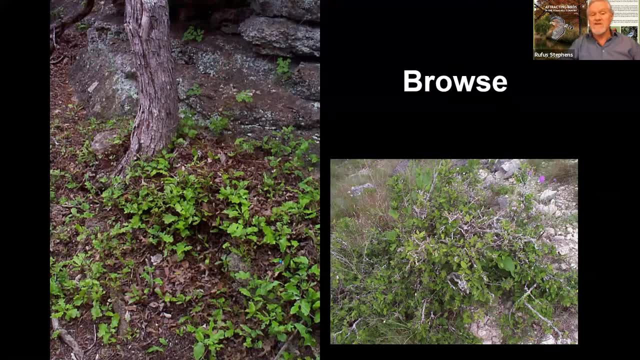 habitat picture I showed of the Kerr area. that was of a chinook thicket And it should have lots of branches of lower growing shoots all the way around it And basically if anybody's familiar with a plum thicket, think of a plum thicket. 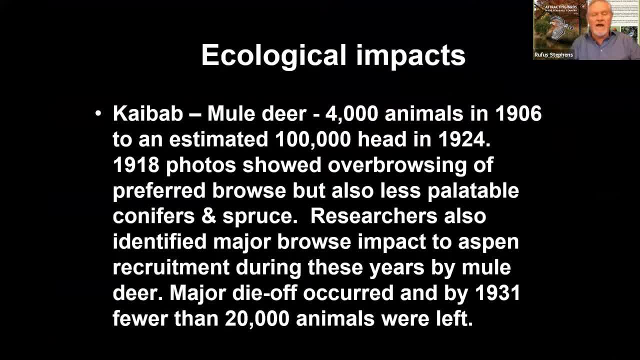 That's what it should look like, not a single tree, Just to you know. you know the ecological impacts. We go back to Kaibab. I mean, I, when I was in college, we talked about Kaibab, which is. 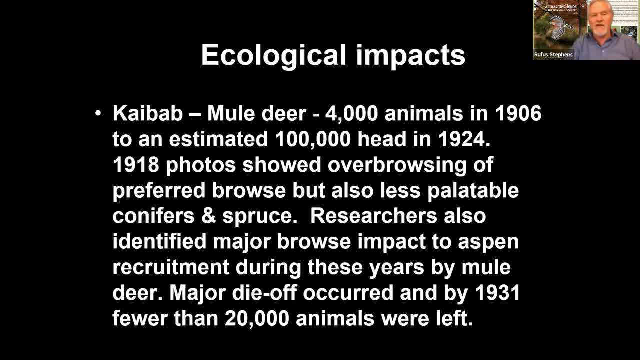 the plateau in Arizona And the mule deer population in 1906 was about 4,000.. The herd, because of controlling predators and such as that, the herd got to and limiting harvest, the population got to 100,000 mule deer. 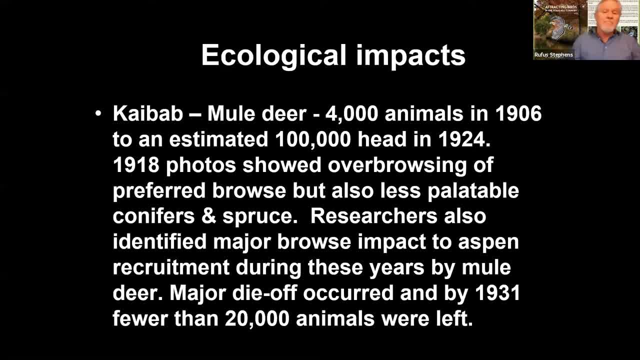 by 1924. And while I don't have any of the early photos showing the habitat in 1918, I do show the area in the 30s and beyond, A major and as it, as it's pointed out, is there was a major die-off in 31,. 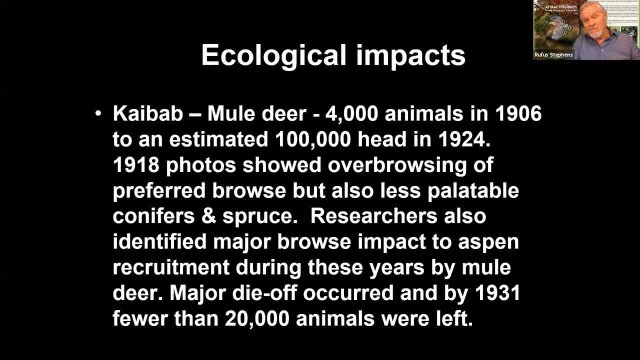 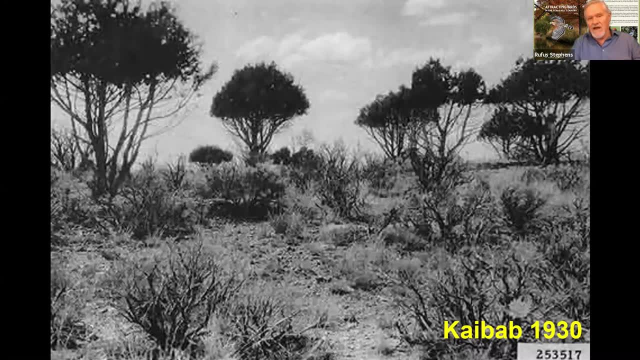 or a major die-off before in the between the 20s and the 30s, And they, the population got, went down to as little as 20,000.. This is the kind of habitat damage that did. Basically, they were standing on their hind, on their hind legs and reaching up. 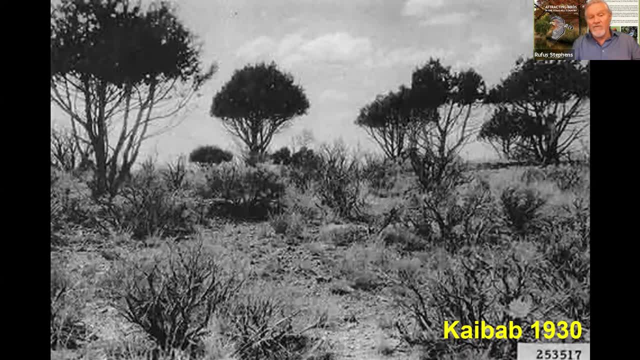 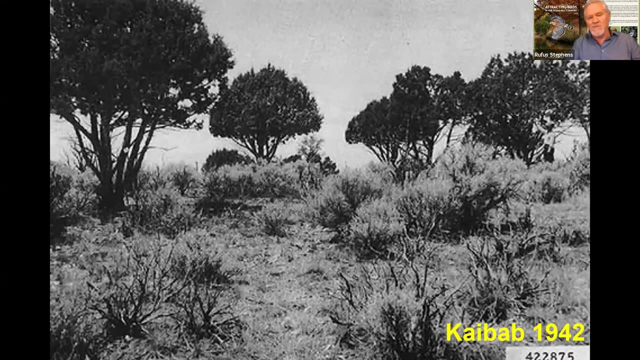 eating these evergreen trees, which is not a really a preferred forage. Much of what you're seeing there that's low, is sagebrush, which is not a preferred food. There's the same spot in 42, is the popular after the population that exploded and and and basically permanently. 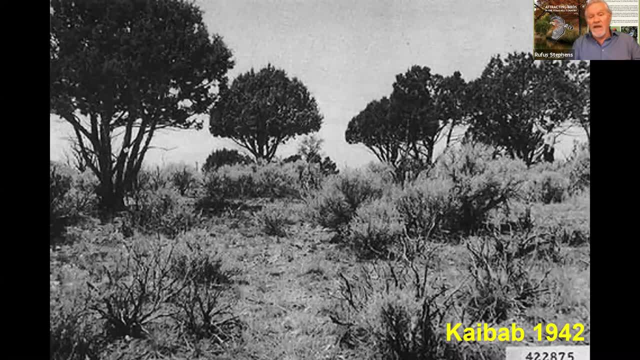 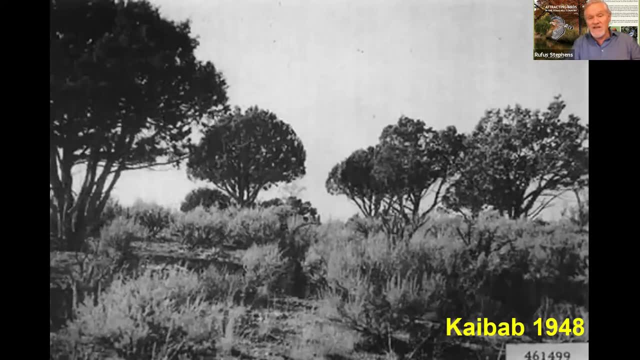 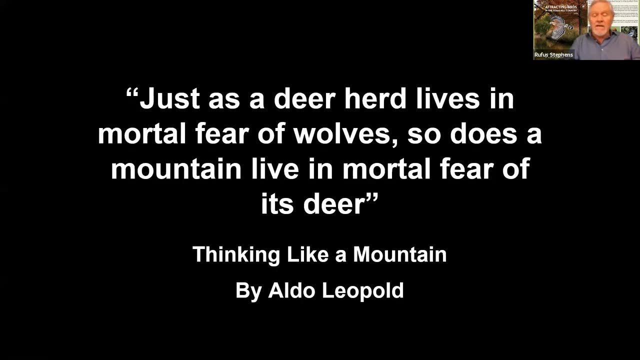 damaged the habitat there And and permanently altered it, And and then here's a picture in 40, 38. So you can see some of that recovering happening at as the after the population had crashed. A great Aldo Leopold quote: just as a deer herd lives in mortal fear of wolves, 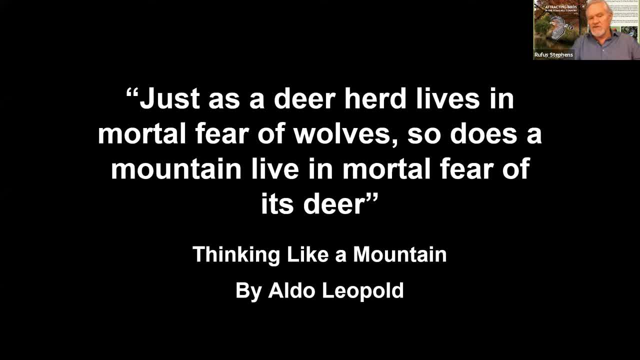 so does a mountain live in mortal fear of its deer, And really that's something we should be thinking about. in the hill country, The, the the impact to the habitat is is dramatic. We look at this and we kind of go that kind of: looks like pretty good habitat. There's some grass. 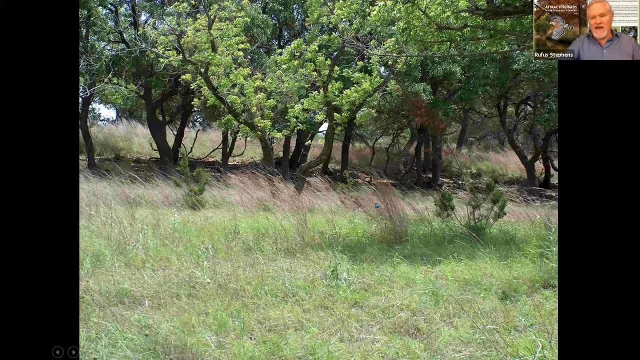 there there's some trees. One of the things that's missing, and actually the only low-growing plants you see, is cedar, And there is a definite browse line here, And all the woody plants are being eaten up to that point. So so sometimes it's kind of deceptive as to the impact that's. 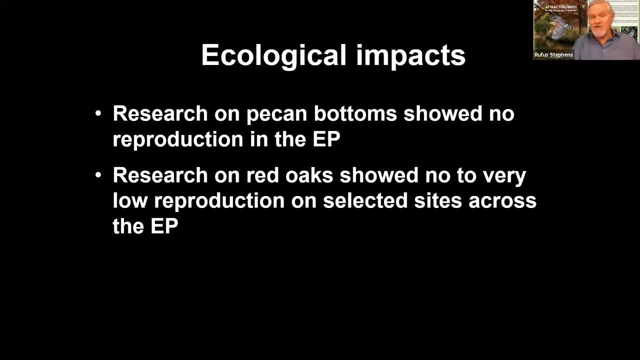 happening. Research in the Edwards Plateau have shown that. you know, there's a lot of you know and pecan bottoms showed no reproduction because of high deer populations. There's other research on on the reproduction in in red oaks And they had. it was either non-existent or very low. 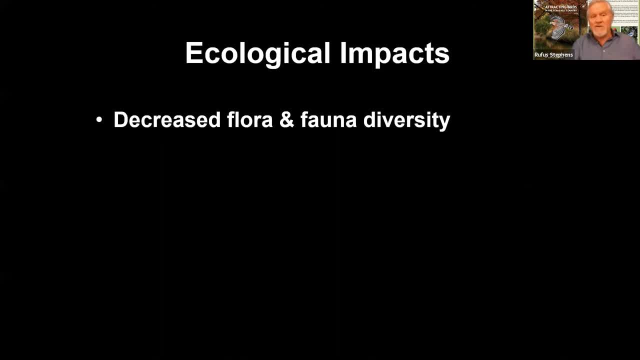 in the Edwards Plateau. So some of these ecological impacts include things like decreased flora and fauna density. decreased wild whitetail deer quality- uh decreased uh. wildlife habitat quality- um uh increased erosion. decreased ecosystem stability, which is 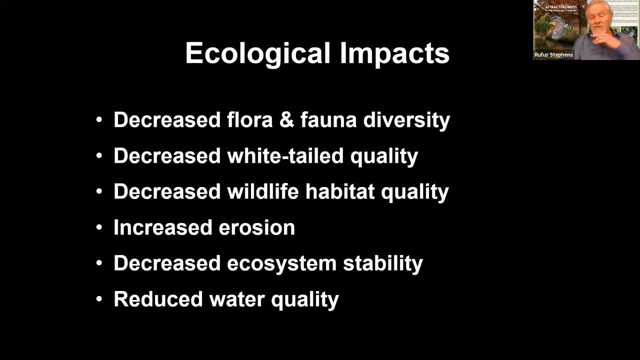 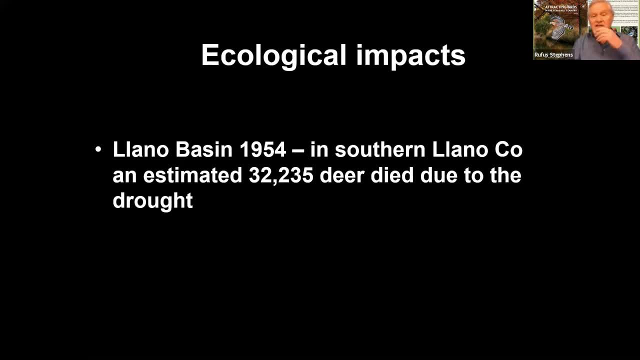 really uh can't be uh, uh overstated at the importance of that Uh. and even reduced water quality. Uh, in the Llano Basin in the fifties there was a a, a huge die-off because of the. 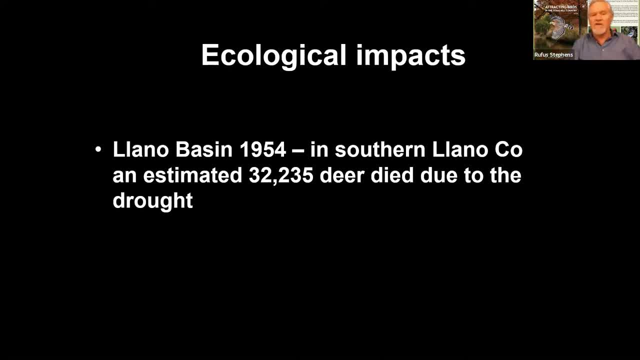 high and basically Llano Basin that's around uh Llano, it's all the granite country north of Fredericksburg around uh Llano And uh it was historically a high deer population area And uh, even in the fifties and actually Parks and Wildlife used to do in the 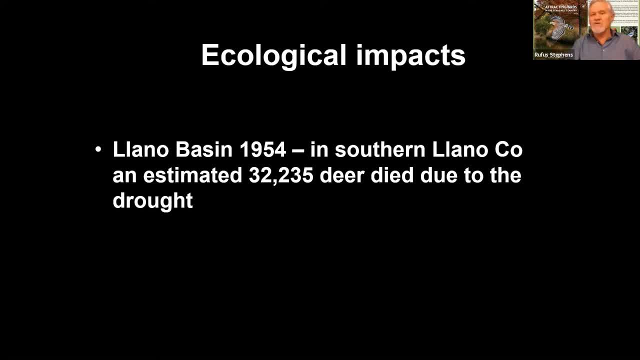 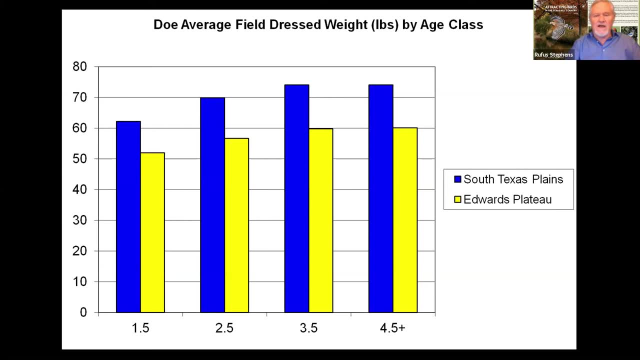 fifties did dead deer surveys. They would just walk transect lines, walk lines and just count the number of dead deer. There were that many dead deer in the fifties. Um, I talked about change in their, in their weights. uh, and you can just see it from the difference between 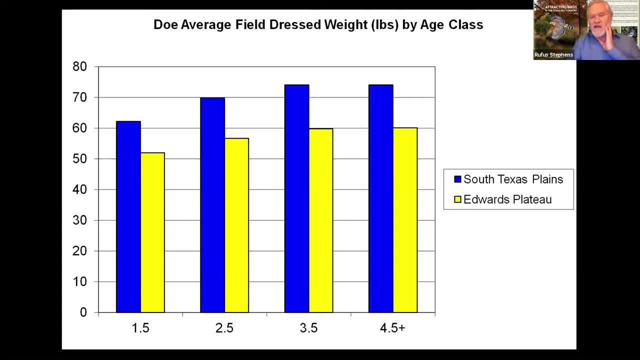 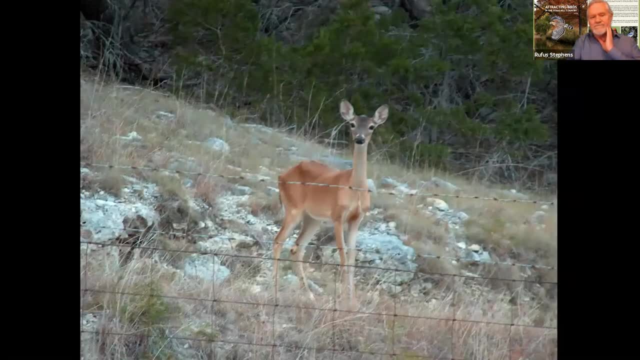 between the South Texas, uh uh, deer and the Edwards plateau, and you go. are those different deer? Actually, the deer in South Texas were repopulated from deer out of the Edwards plateau, So they're genetically the same deer. uh, at least now. Um, you know again, very uh uh. 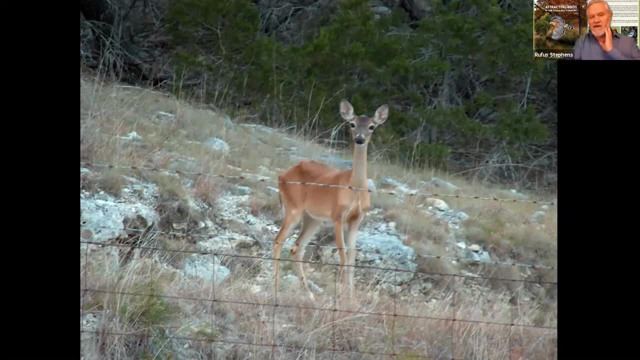 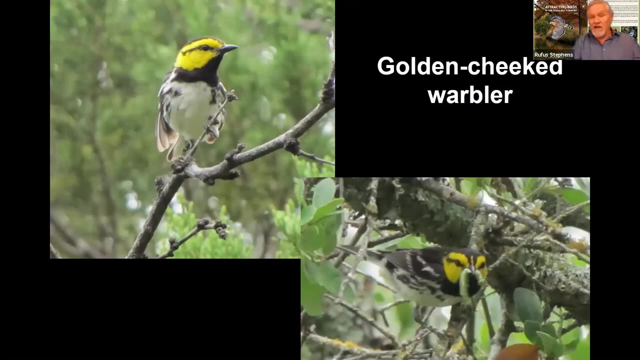 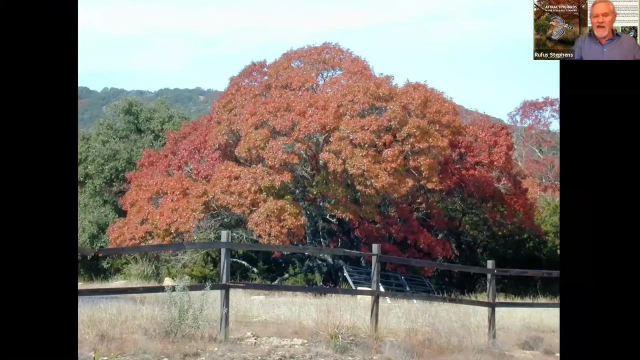 poor quality, disturbed, disturbing looking uh health of deer because of the poor quality of the habitat Uh things and the impact to other types of wildlife. so golden cheek warblers, they are a. they need cedar, but they also need uh spanish oak. that is uh an important component of good um uh golden. 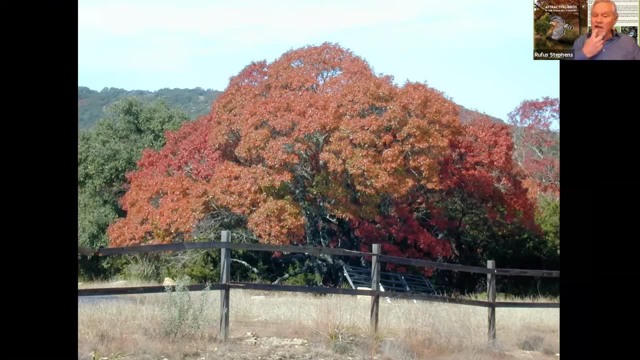 cheek habitat and if you, uh, and one of the things that we or i talk about is that really we're headed for a slow train wreck, because what we don't have is any reproduction on spanish oak because of the high deer population, um, for the past, uh, 50 years, so, as these trade trees age out, 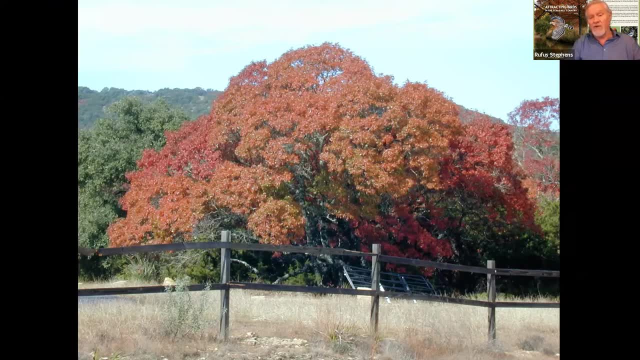 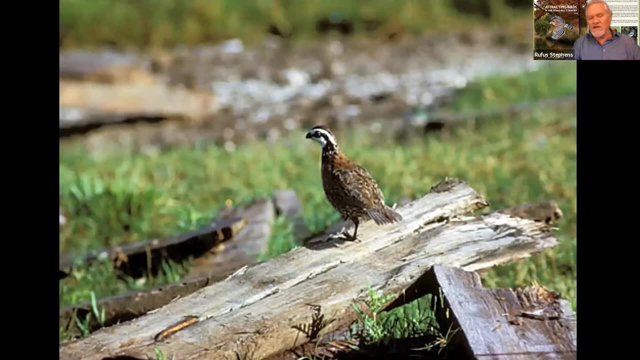 uh, there's not going to be any replacement trees if our deer population stays at the level it's at. other species- bobwhite, quail- are impacted because of forbs- right, that's, that's the food for for quail, those seeds from forbs, um, but also these species which uh tend to need low, uh cover uh. hermit thrush. 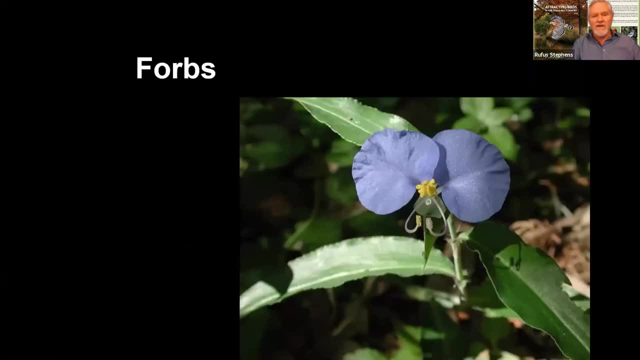 spotted uh tohi and louisiana water thrush. um, you know, we, you know i already said about forbs and we can kind of see how that uh, and this is dayflower which is actually makes it is a great food for uh quail, but deer love it. um, but also uh. well, where do what? what else do? 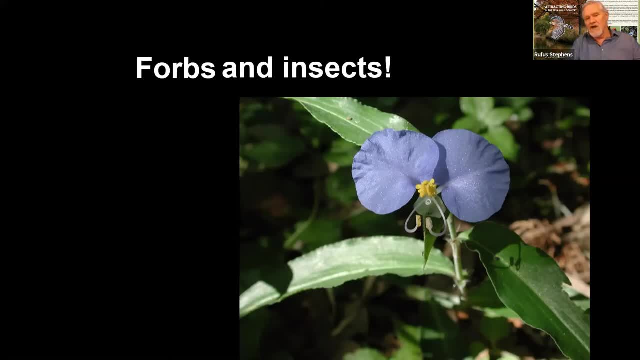 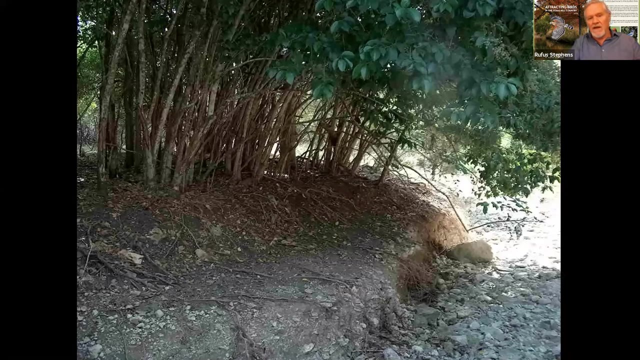 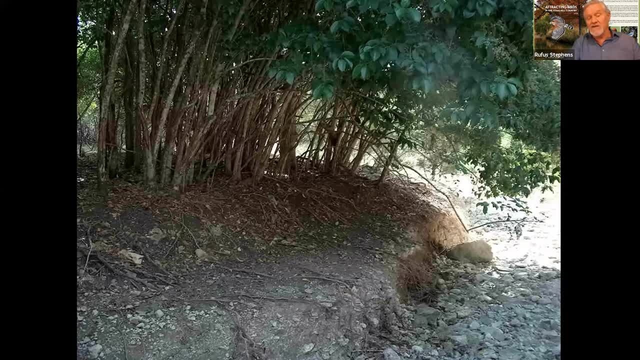 this is axis um, and it's actually this community. this stream has changed from having native vegetation on it to ligustrum, to an exotic plant, uh, and then another exotics coming in and putting a browse line on the ligustrum, um. but you can see that this is not healthy situation. we're having erosion going on, uh. 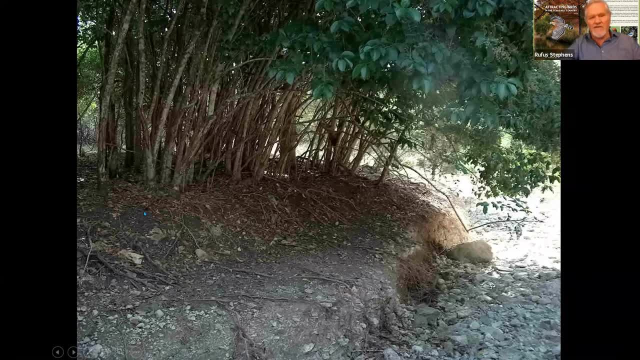 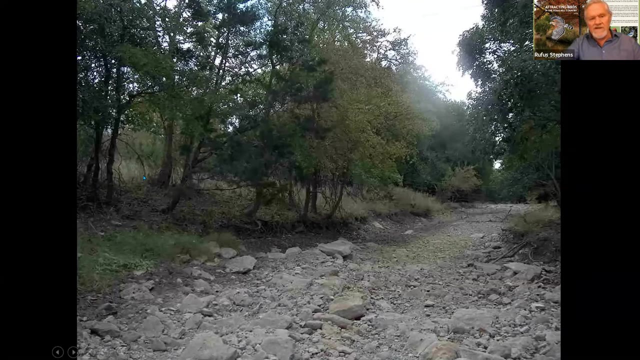 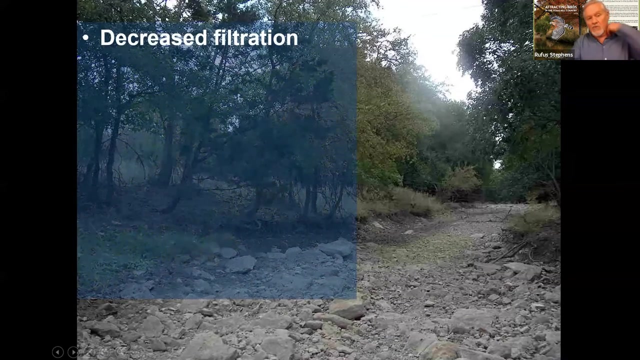 there's an unstable bank here. uh, there's not a very low diversity. that's actually not only because of the animals, but also because of the exotic plants. uh, and here's another shot. so browse line clearly on this habitat and active erosion going on here, um and uh. so what can you know? as i mentioned, 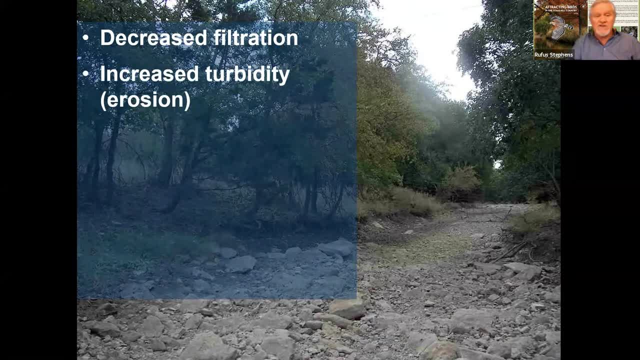 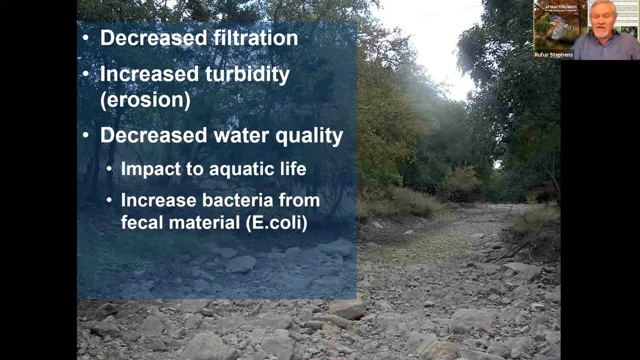 water quality. so this increases uh turbidity from this erosion uh, and so that decreases water quality and it'll impact aquatic life- we kind of don't think about deer impacting aquatic life in that way uh- and then also increase bacteria from uh, from fecal material e coli. 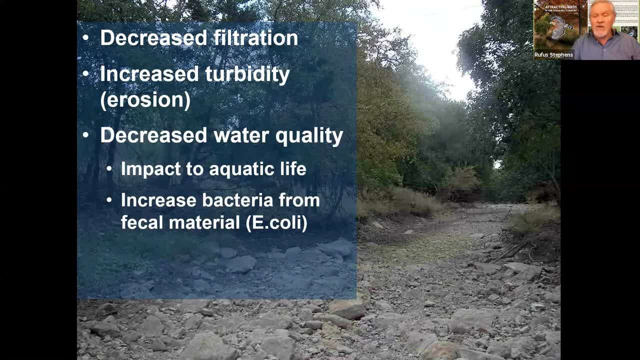 basically, and uh that has actually showed up in a number of uh watershed protection programs that they look. they're looking at the number, the deer populations in their watersheds and how that contributes to high e coli levels. um, and then uh, decreased base flow uh of a stream or a riparian. 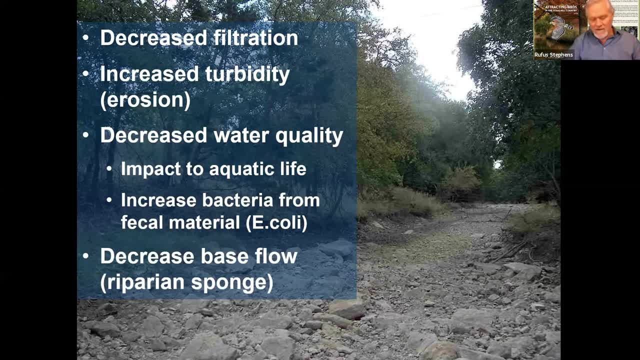 area, the riparian sponge. if anybody's seen uh uh or heard um um steve nelly, he talks about the riparian sponge and this lack of vegetation along the shore, along a creek bed, is where that riparian sponge should be and is not because of all the the over. 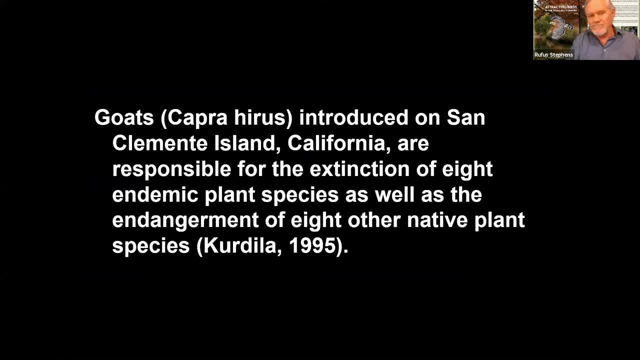 browsing um just in and on the uh san clemente islands off of the california coast, um goats that were introduced um cause of these overgrown plants. um. so these are- uh these are still in the bottom of the reinventing wheel. uh, we still have more of these ready to come into use later on in a. 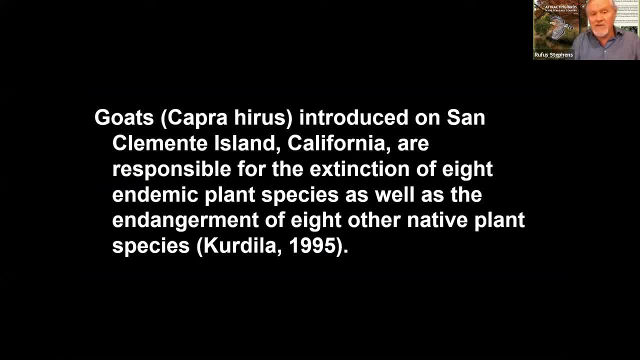 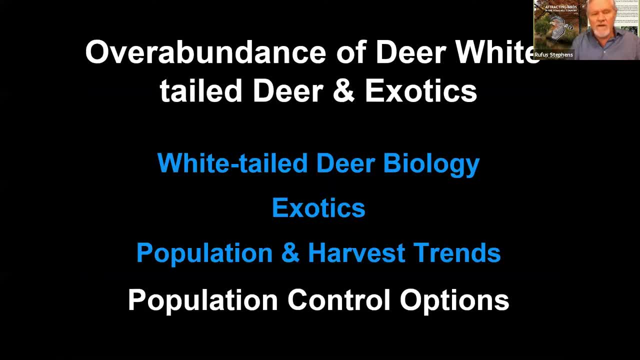 responsible for the extinction of eight endemic plants. meaning endemic means they only occurred on those islands and endangered another eight more. So we've kind of made a case for why we need to be concerned about high deer populations. What are the options? Basically, those options. 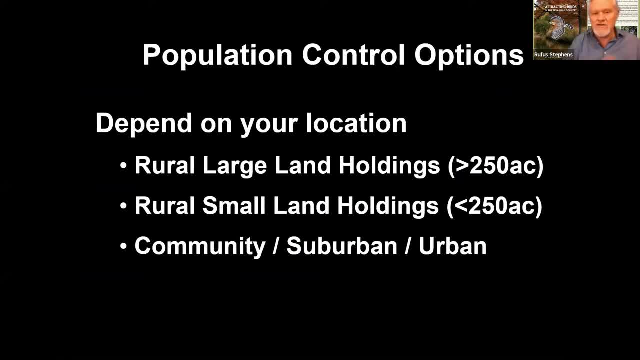 depend on where you're located. So rural large landowners more than 250 acres, they have a set really options that smaller acreage landowners don't necessarily have. So rural landowners that are less than 250 acres those are. there's more limitations to what they can do, Not so much from. 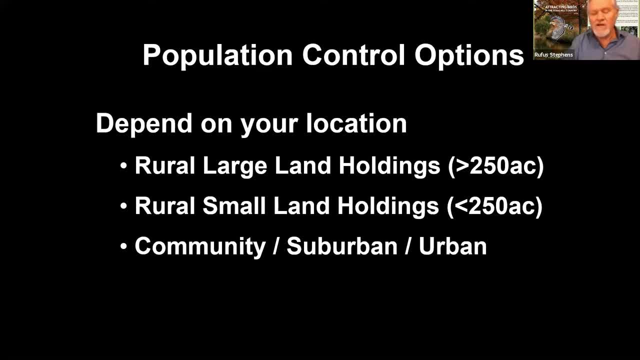 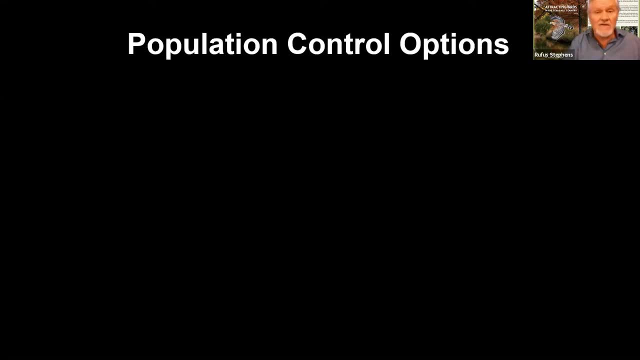 a some from a permit standpoint, but more so from just being able to safely harvest deer and such as that. But then you know, then we talk about suburban, community, urban deer and that that is another challenge right there. So what are one of the some of the things? Well, 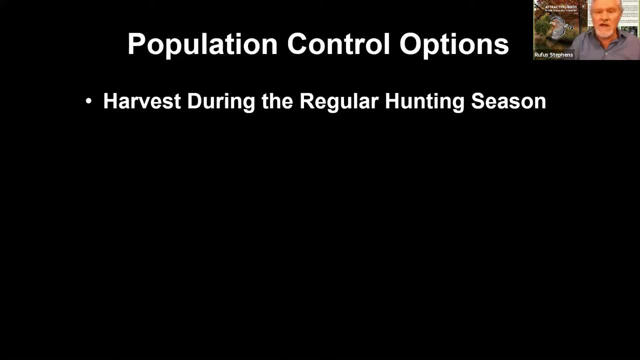 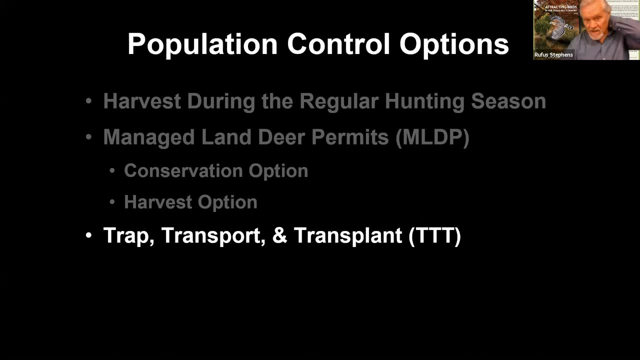 the basic one is harvesting during the regular hunting season. There are managed land deer permits- MLDPs- and there's two different types. There's the conservation option and the harvest option. Then there's permits that Parks and Wildlife does that are called. 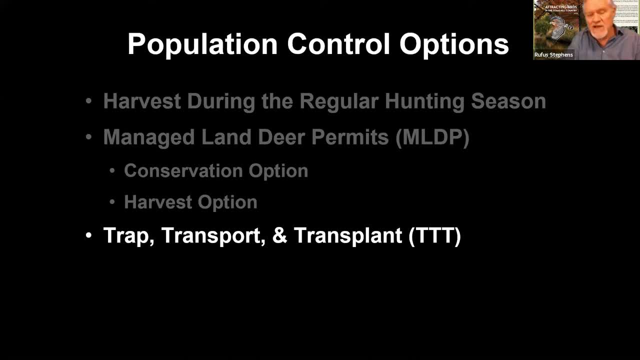 triple T's: trap, transport and transplant, And basically it's: it's trapping deer, moving them someplace else and letting them go. Problem is is there's no place, there's almost no place that in the state where they don't already have too many deer, And so there are very few places that. 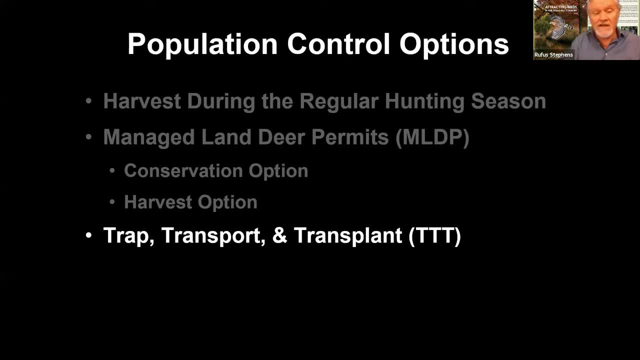 Parks and Wildlife will approve a relocation like that, And that's why they got into what was what's called the trap, transport and process, And basically that's trapping them, take them to a slaughterhouse and then processing them And then they have to be donated for, for food banks or for. 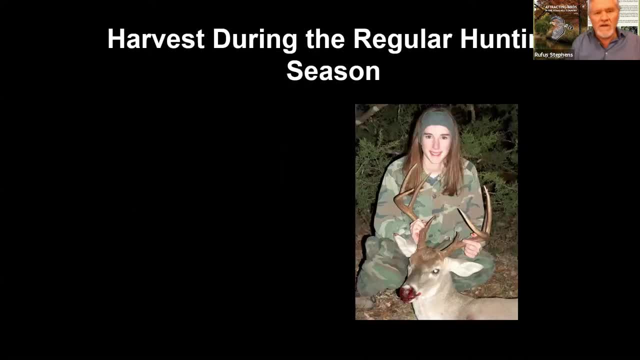 non-profits that are feeding the hungry. So hunting during the regular season- You know TP- just for an example, TPW regulations for Kerr County- allows up to five deer to be hunted And then they have to be donated to a slaughterhouse And then they have to be. 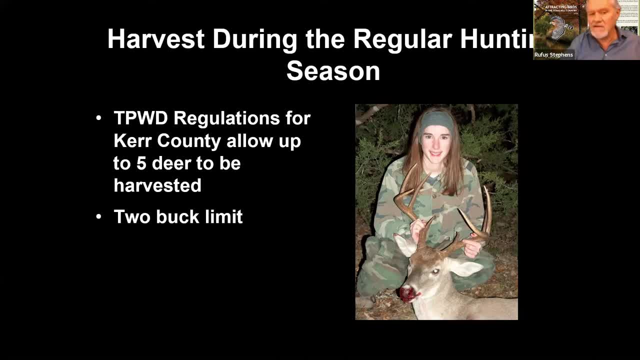 harvested And it has a two buck limit. So you could- you could- shoot five does, and or you can shoot four does in one buck, or you can shoot three does in two bucks, but you can't shoot more than two bucks, And that's pretty much the regulation for all the surrounding counties. 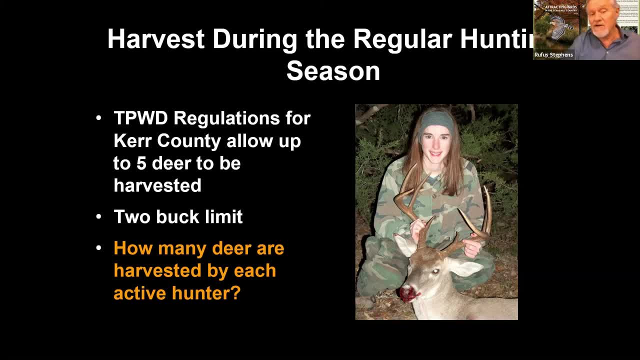 around Kerr County. So how many deer are harvested by each active hunter? And I'll let y'all- some of y'all have seen my this presentation before and so you know the answer. The answer is about one, and a little bit more than one. 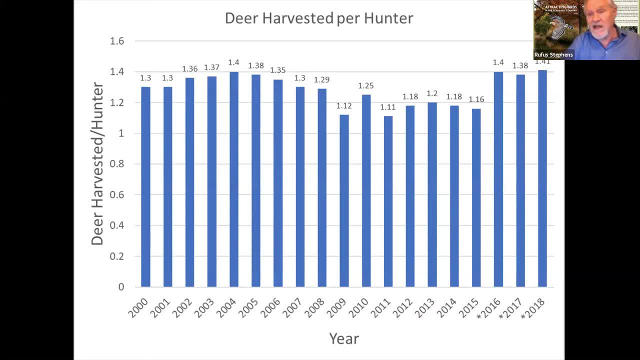 So you can look at basically the last 20 years of data and the highest it's been is like 1.4. And so hunters are not shooting more than one shooting more than one or one and a half deer per hunter on average. So that means some active hunters are shooting none. 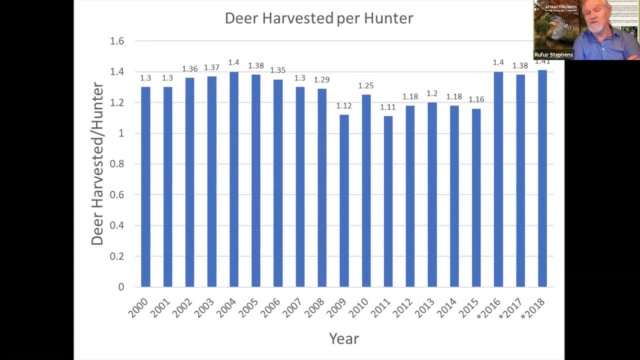 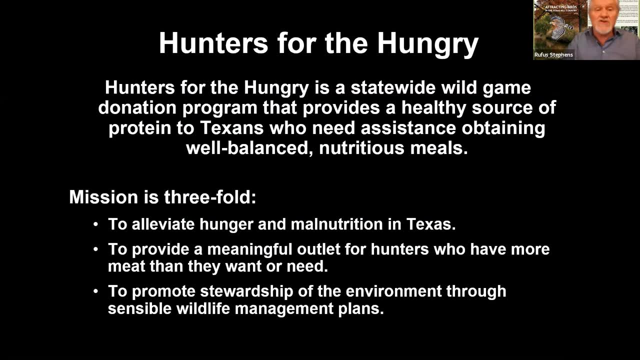 some- a few- are shooting more, but most hunters are shooting around one. That's probably pretty typical, but they can shoot five and they don't. So one of the things is Hunters for the Hungry. It's basically a statewide program for donating wild game. 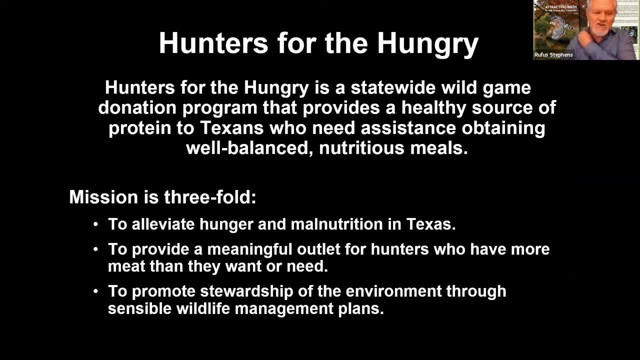 And it's. it's primary mission is to alleviate hunger and malnutrition in Texas and provides an outlet for hunters who have more meat than they want, And it's promotes stewardship of the environment by increasing the harvest. So these go to go to, basically, food banks. 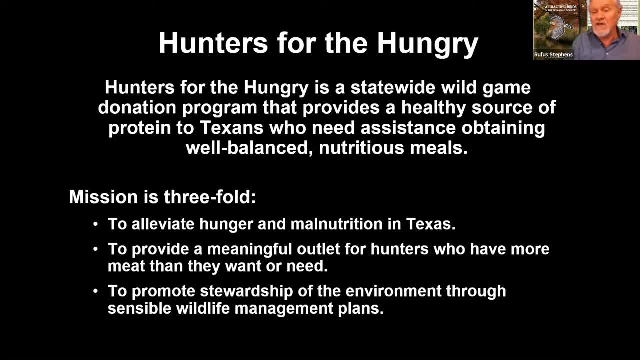 And so most- a lot of processors do this. It does. there's a fee associated with it for the basic processing. They basically turn everything into hamburger and then they give it to food banks- and actually food banks really need this. A good source of protein is something. 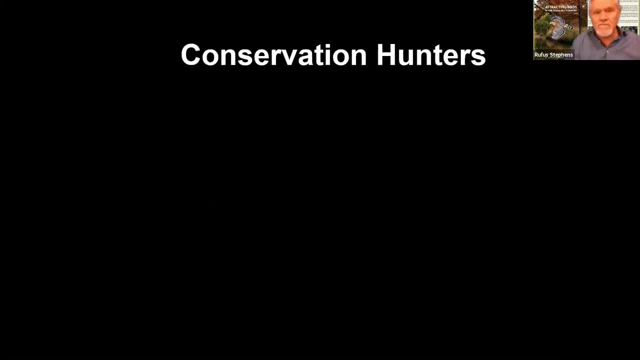 they really don't have. So another concept is conservation hunters, And I talk about this and kind of have coined this, and conservation hunter is basically a hunter that harvest to improve the overall herd health, And they do it also to improve habitat health And they're also providing it's more subsistence. 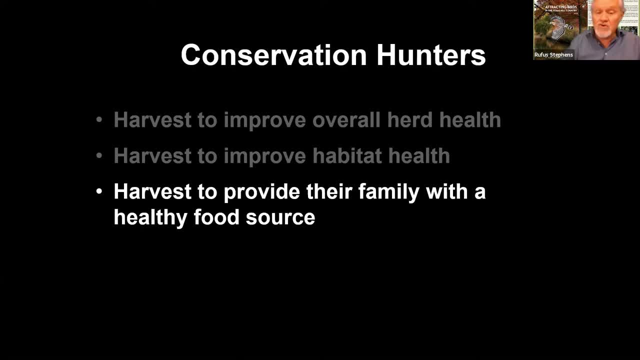 They're providing a a healthy food source. So when we talk about local vores or being a local vore and and eating local sources of food, there's nothing more local than than harvesting meat from, for axis or white tail deer. 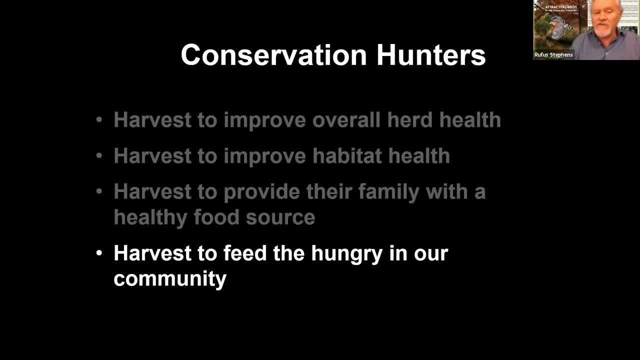 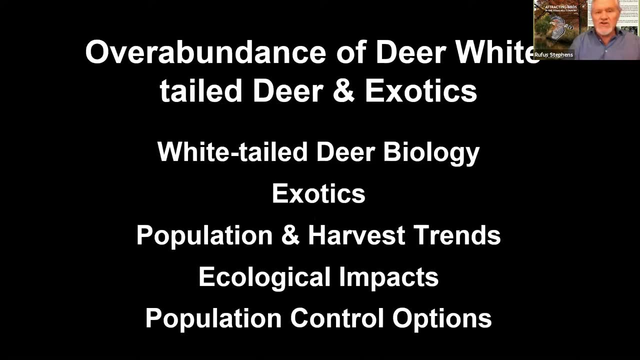 And then also they harvest to feed the hungry in our community through programs like Hunters for the Hungry. So basically, I talked about the overabundance of of deer, of white tail deer and exotics. I talked about their basic biology, some of the population data that we have. 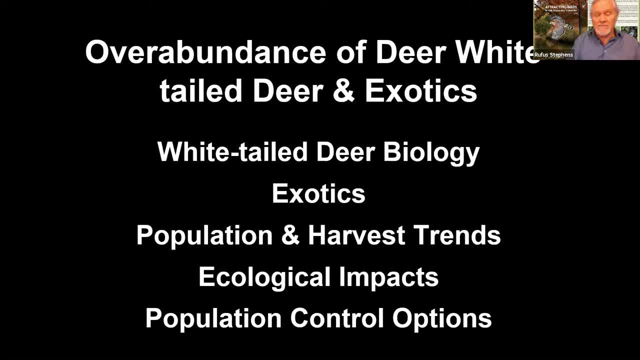 the ecological impacts, And then I talked about some of the control options. So let's let's start there, And I think that hopefully, I what I should have mentioned right up front was that if you got a question, we can put it in the chat. 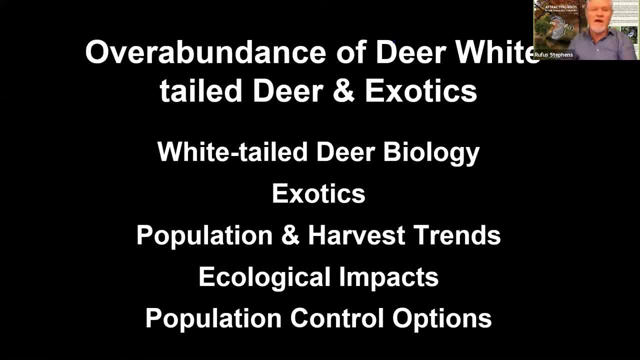 or we can just I'm I'm happy to open up a discussion And I think that Darrell was maybe going to help me with some of the chat. If there there are any questions, we can put them in there about any part of my presentation or on the. 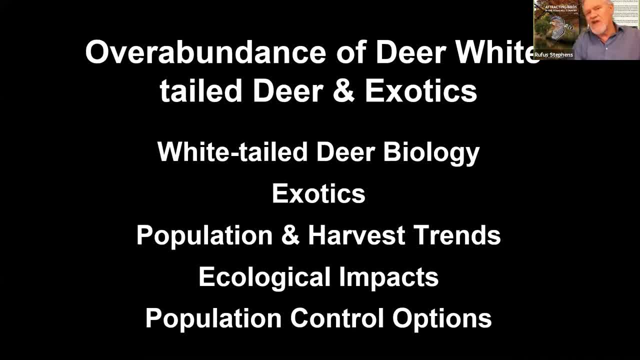 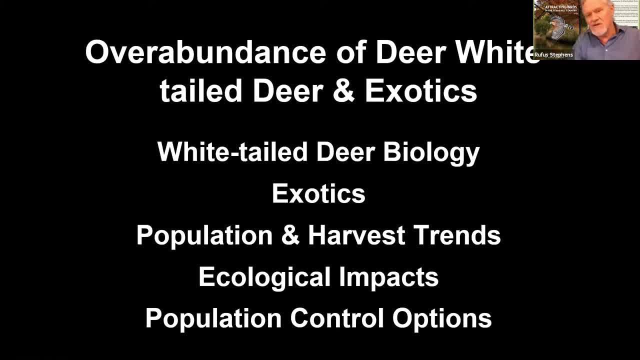 I don't know, I don't know, I don't know, How long do we the challenges? so how do we manage deer populations when they're so high Rufus- It looks like we have two questions in chat right now. 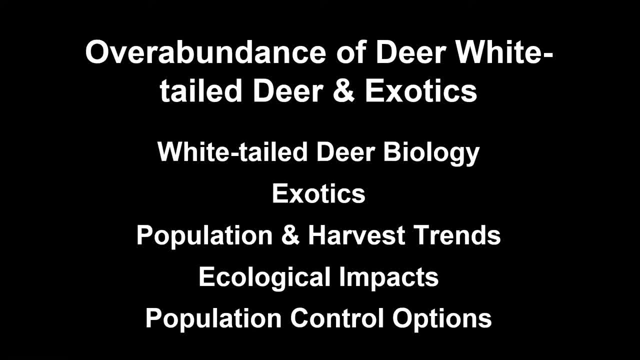 and one of them is from Elsa And it was. is there an increase in trophy hunting that has increased the buck harvest? So that's a good question. So trophy hunting is- so? in Texas, subsistence hunting was really in the early days. that's what people did. 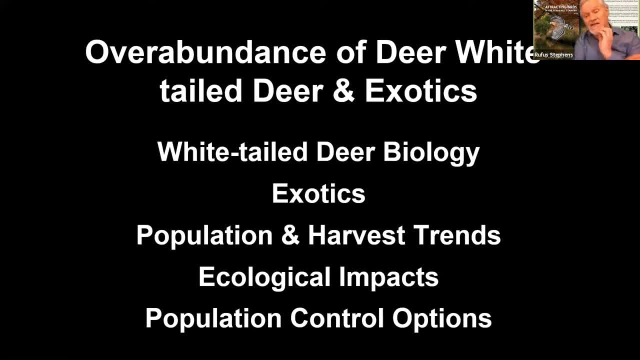 And then in the early part of the 1900s of the last century it switched to market hunting And there was actually 175,000 deer hides shipped from Austin to back east for making into handbags and stuff in, like the 1920s. 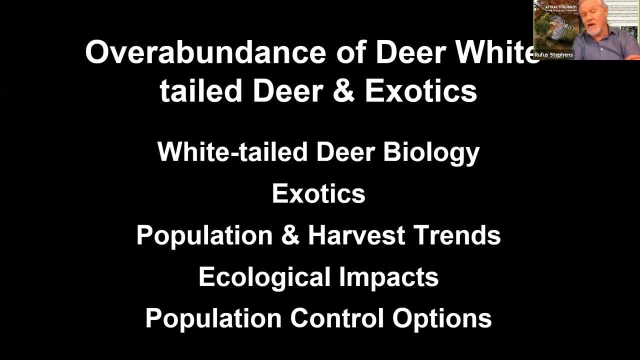 Then we began to do regulations, then trophy hunting became a thing, And because what we wanna do is, if we're trying to control the population, we need to control the breeding side of the population, meaning the doe side. sorry, ladies, but they are the ones that really control. 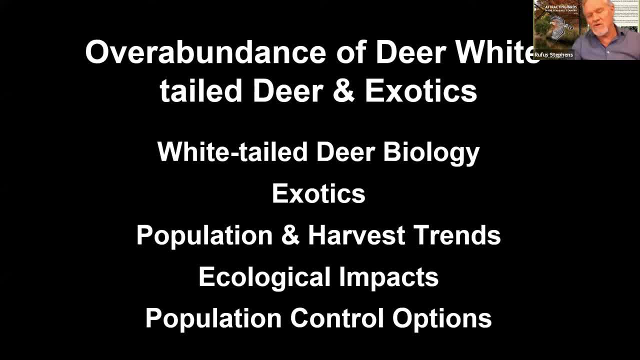 the That the population control is related to. So if we shoot more bucks, one buck can still breed numerous number of does, though it doesn't help us to harvest more bucks. Our population data and looking at the trends, remember mainly it's about half and half. 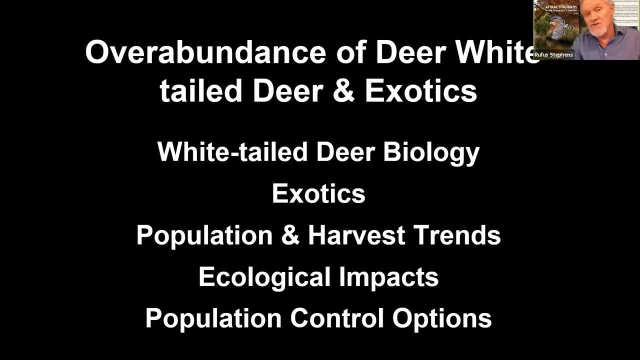 and even it's increased a little bit on the buck harvest. So most of the deer that are harvested- at least half of them- are bucks and not does, which is really what we need to do in order to control the population. So how do we increase that when we have that? 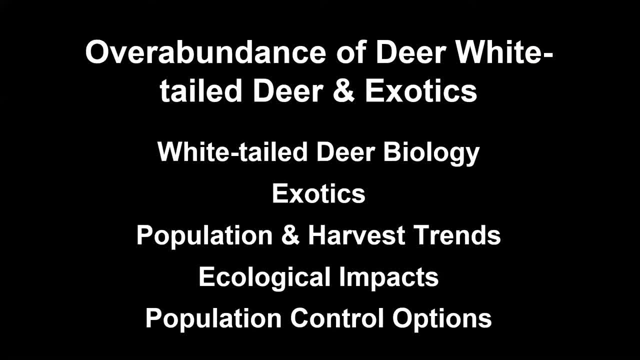 So I have another question from Anne Ryan. She asks: can you talk more about the riparian sponge? and what is it? Okay, sure So, the riparian sponge so when you have a vegetation that's growing on the edge of a stream, so riparian is streamside habitat, When you have 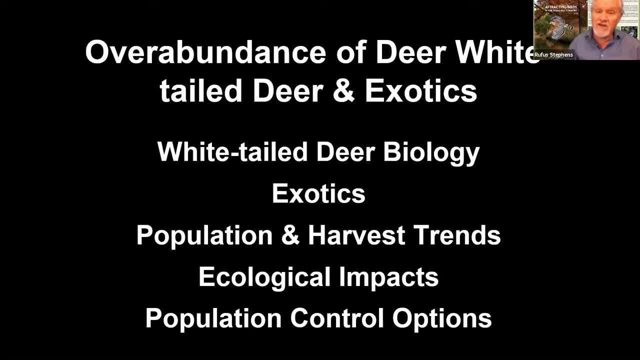 that diversity of vegetation that's growing on the edge when we have higher flows. those plants help to store and hold water within their root systems and then slowly release it to the stream over time, And that's what we talk about when we're talking about the riparian sponge. 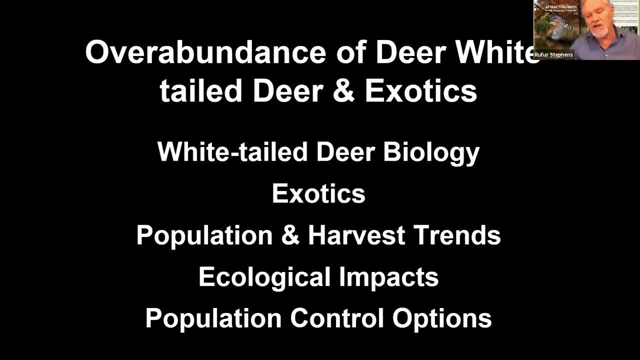 So it's a way that the plant community holds water and allows it to be released- shallow water- and it allows it to be released and sustains that stream over time. If we lose that vegetation, then the stream becomes much more drought prone and so will dry out faster. That's a good question. 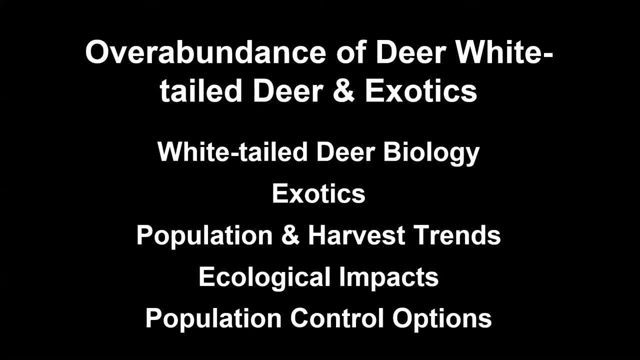 So I have another question from Lucy. She asks: is there any type of deer sterilization done in Texas? That's great, That's a great question. So in Texas, Texas Parks and Wildlife would be the ones that would have to authorize it. So deer sterilization. so there's two things related to deer sterilization. 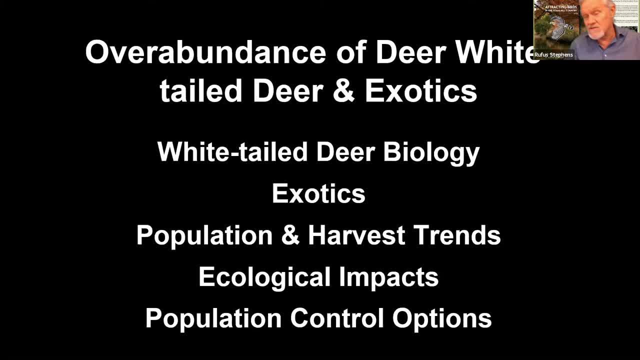 One would be physical sterilization through surgery, The other would be through birth control, And so for birth control it's not currently allowed in Texas. There's no permit permitted, other than for research. There's been some research on it And currently there's not any good. 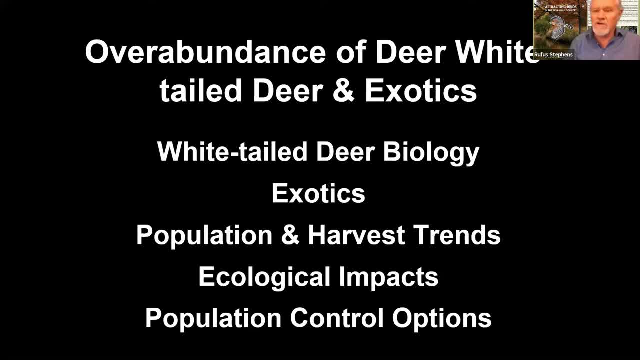 birth control for deer. The problem is that, just like with people you have, you know it's either managing testosterone or managing estrogen, And so it's a sex-specific kind of treatment. So they need to be given to the dose. So that's why you can't just put a feed laced with some type of birth control in it. 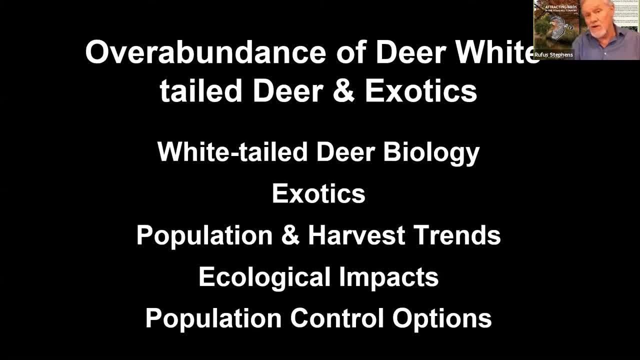 And it needs to be dosed properly in order to work well, And the way that it has been done in the past has been using a. the products that are Spavac that has been used in the past has a. the problem is is that you, you, you- have to give them a shot. 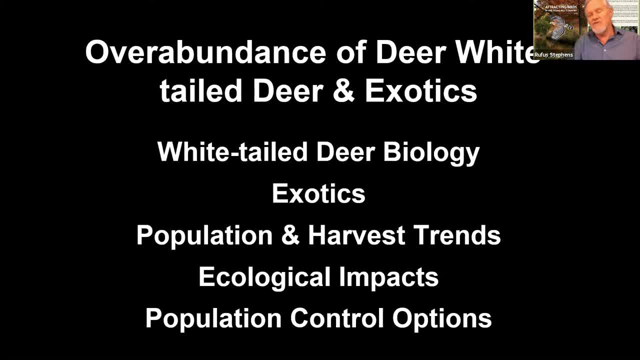 You either need to trap them or you need to dart them. But even if you dart them, you have to- uh, you have to go back and give them a booster, Otherwise they do not. they're not successful, Kind of like our, our, our COVID vaccine. But uh, they are, it's, it's. 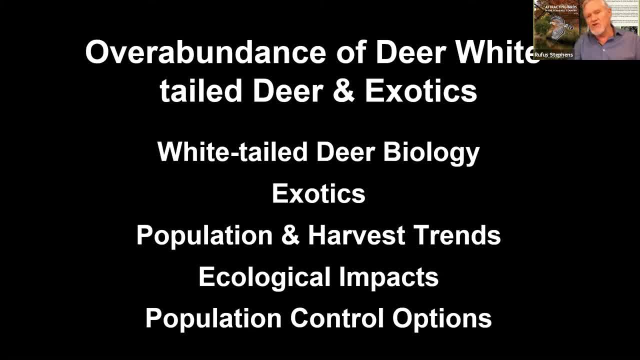 not as effective, uh, without the booster. So that means you got to somehow identify the deer that you've treated and then go back and retreat that animal It is. that is extremely difficult. It makes it very difficult, And the same is true of trying to to do a surgical sterilization. 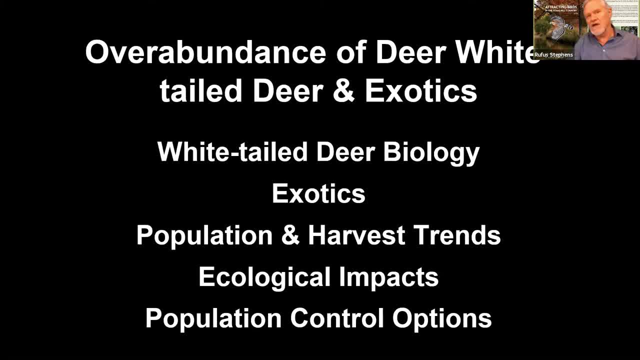 um, there have been on very small, uh like research facilities where they've been able to do that. But the problem is: is being able to capture enough of the deer to be able to do it? Now we have there's a dilemma. So if we sterilized half the deer population, uh, if, 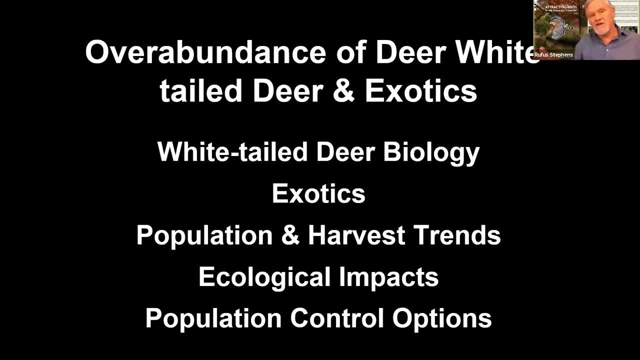 if um the um because the, the they're in such poor health as as health increased the number that are still left out there, they're able to reproduce, are in better health and can have more fawns, So we will end up with a rebound in the population. 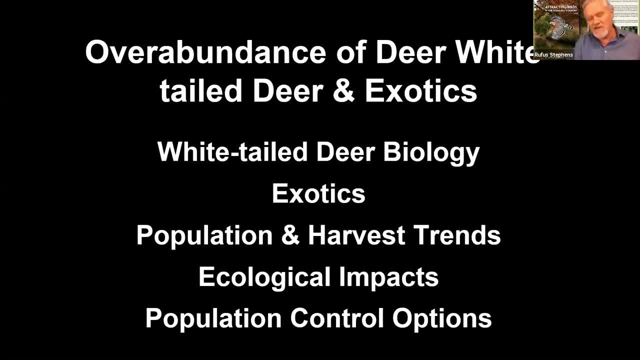 even though we've treated a large percentage of the population. There was uh some research done on Johnson Space Center, So it's a high fence property uh obviously down there, uh in outside of Houston, And they, um, and it was they- realized that they had to get uh somewhere around 70% of the population. 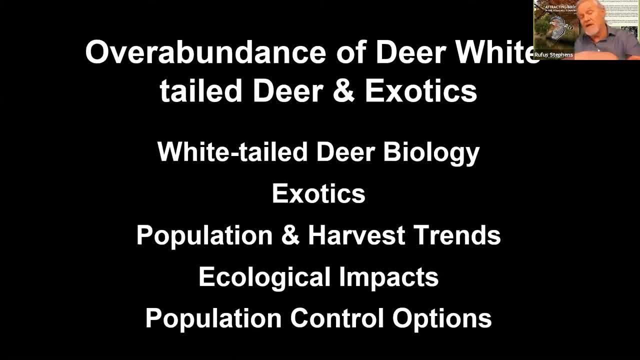 to be able to all this, to have the populate treat 70% of the population, to have it begin to decrease, So that's an incredibly hot high bar. So that's the reason that those techniques have not been uh successful and are extremely problematic. 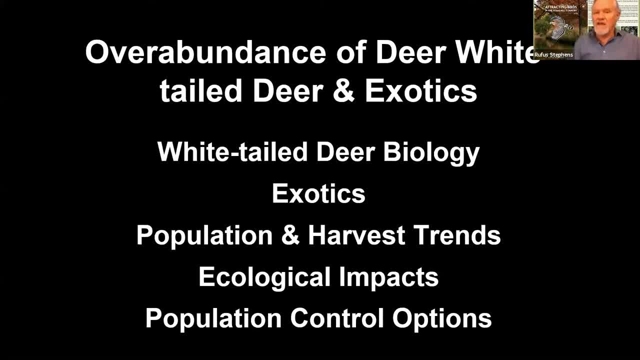 Now we may. we may get into the future where we have a more effective, less um uh sex specific kind of of uh birth control, And that would really go a long way to potentially uh taking care of the population. But that's um, there's nothing on the horizon right now. 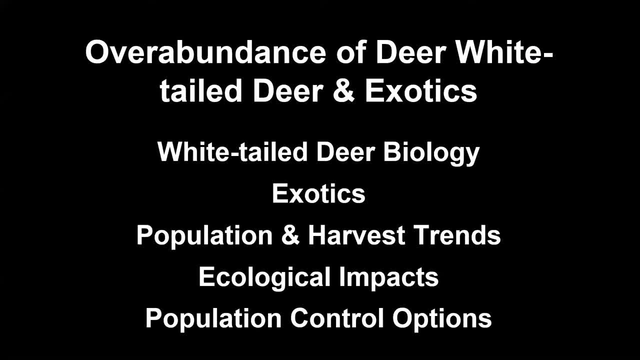 that I know of. So I have a question from Jeff Schwartz and he's asking: uh, what do you think the freeze did for you? What's the advantage to the deer population in the Edwards plateau? That's a good question. Actually, I think it will probably impact the access population. 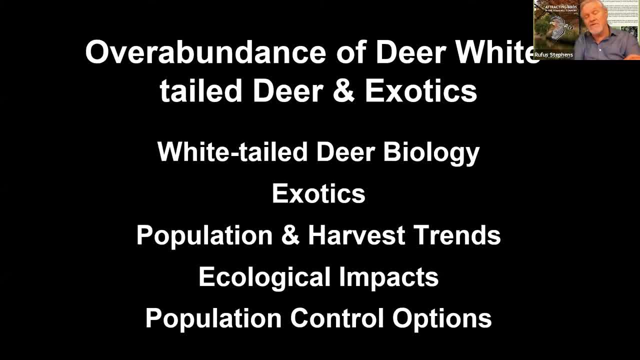 more than it'll, because they're really a more of a tropical subtropical species than is whitetail deer and whitetail deer are more adapted to that. Uh, we certainly uh. in the past we have seen uh with, um, uh, very cold, uh, cold snaps. I think that in 2011,. 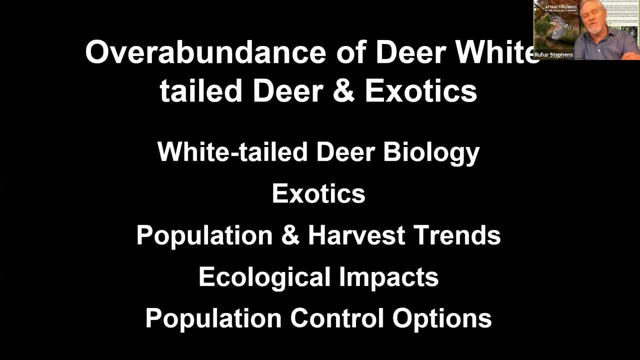 we had the last Pretty good cold snap, ice storm. We had uh that, that, uh that we lost a number of deer, but it's, you know, it's a blip in the overall population. Um, one of the things, too is: 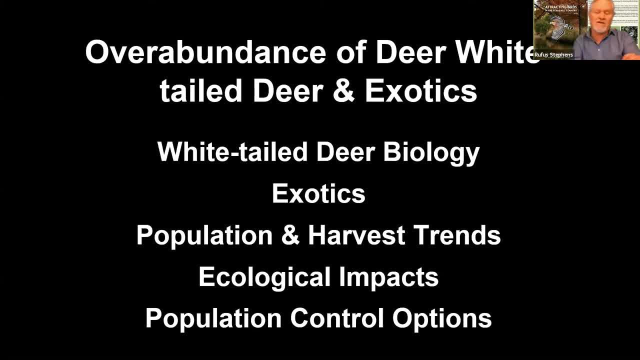 uh, I'll go ahead and bring this up as part of the discussion. So, um, we, so, uh, you know what was the control mechanism. I mentioned predators And, uh, you know there's, there's. 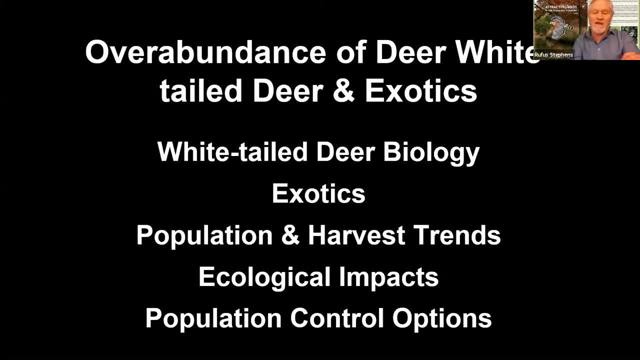 there's a lot of control mechanisms in with Kaibab, but uh, in Texas, uh it's- we probably never had enough uh wolves or um mountain lions to control the deer population, And really the hill country was more prairie And so it wasn't very good deer habitat. So 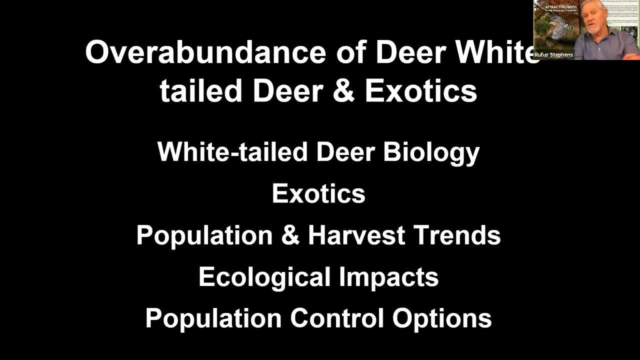 it's mainly bison, and it was even antelope in the hill country, uh, which says how open it was. Um and. but there was another control mechanism, And that was screw worms, And anybody who grew up in the hill country or grew up on a ranch in Texas is familiar with screw worms. 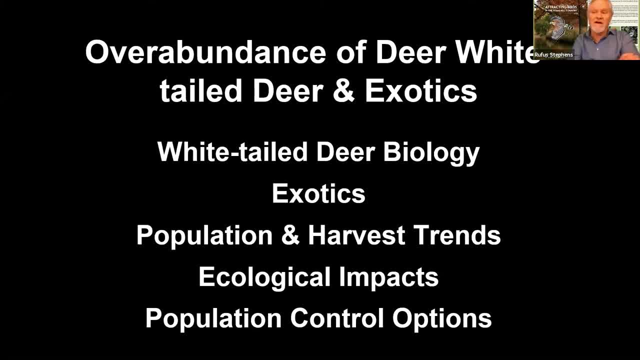 And they're an insidious critter and they basically lay their larvae in an open wound and it caused significant amounts of mortality in deer populations And basically we controlled screw worms for the livestock industry by releasing sterile males in the population of screw worms crashed. 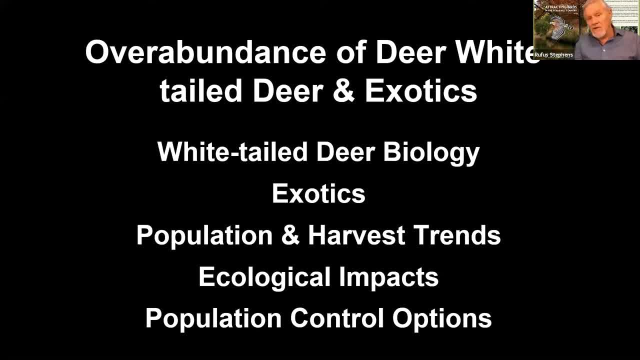 There's still screw worms in Mexico and we continue to release sterile flies to maintain a low screw worm population in the United States. But it happened. It was a significant- it was the most significant, probably- mechanism on controlling deer populations And when that changed was in the late 50s and early 60s. 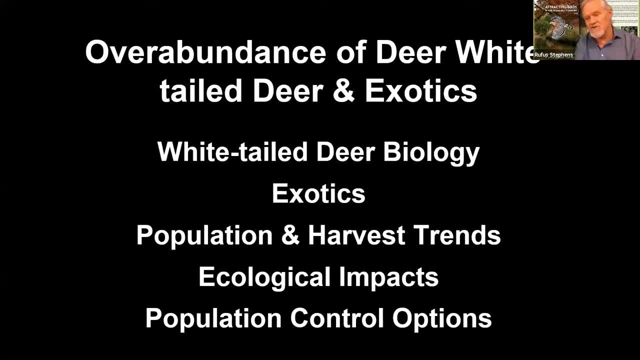 And that's when our deer population just takes off and just goes sky high. So that was the control mechanism. I don't think ranchers want us to bring that back. I don't think policy makers will allow us to make that come back. 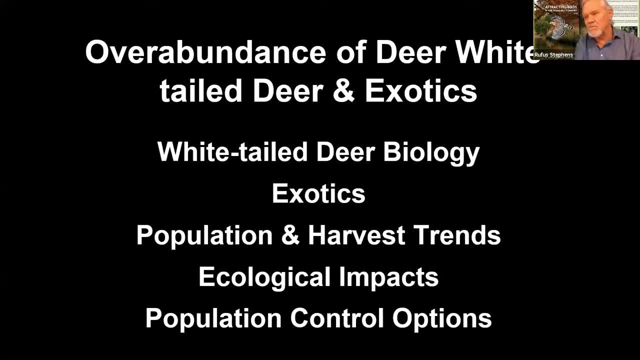 But it's important to understand that the predator problem, The prey relationship, It was really a parasite And, you know, a pest, that that controlled the deer population, not not mountain lions, not not wolves. We have lots of coyotes and they are not having a control on it. 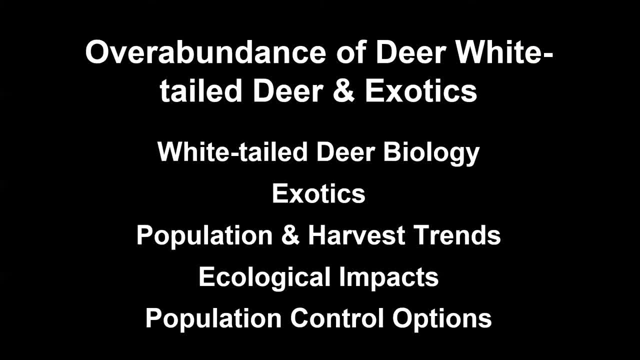 So I had a question from Gary he would like to know is why not open hunting season to all year? That's it Now. that's a great. so now we're getting into the good, good part of the discussion. So, um, that's a good question. So we do have like with access deer, and access deer, probably our most numerous exotic and continued to the population, continues to grow. 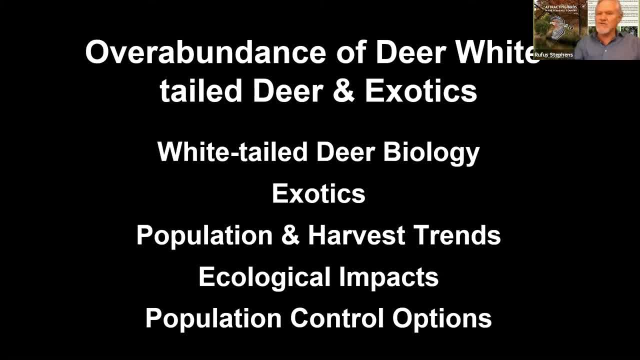 We do not have a closed season on access access. you can harvest year round. There is no bag limit. You can. you you're not limited to five. you could shoot it. You can shoot 20 in a day. you could do it if you wanted to trap access. 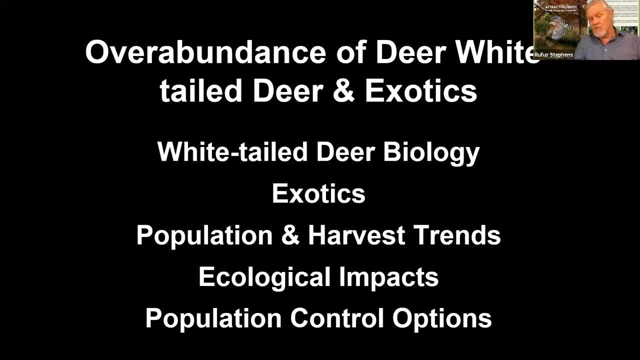 And sell them. You could do that. You can't do that with whitetail deer without a permit, And so so there was: there's no bag limit on access, There's no closed season on access and we still are not removing enough to control that. The other thing is: is actually hunters? 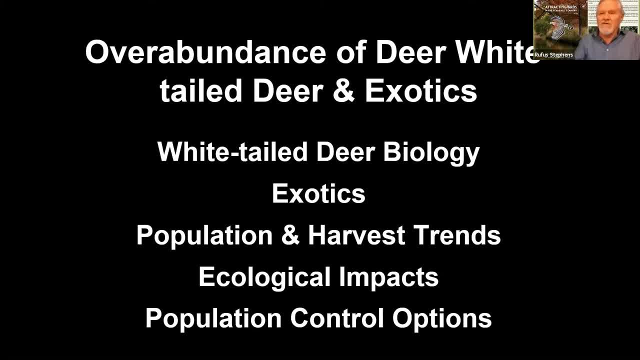 They are very uncomfortable with the idea of harvesting deer when they think They may be. You know when they when they would have a sizable fetus in them. So they're not comfortable with doing that. And even if we show, if we, even if we did have an open season year round, It's doubtful that there would be any significant harvest. 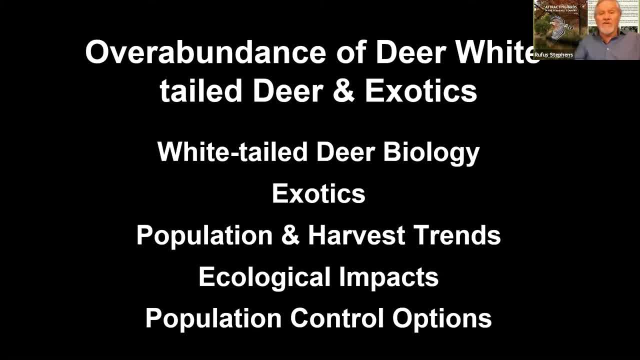 You know from you know another month or two from now till the end of, Probably until the end of, Middle September. The other thing is is is hunters also do not like the idea and they are concerned about whether a fawn can survive. So a fawn can actually survive from a 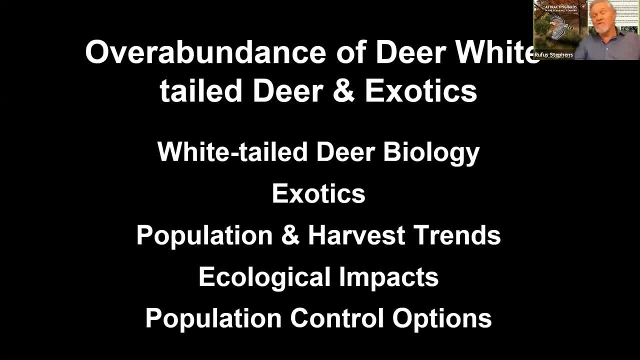 doe from its- you know, being weaned from its doe at about 60 days. So most of them are born the first couple weeks of June till first July. We get some late ones, Usually they're. We get some late ones that have been bred, So they were yearling or they're actually not even a year yet and they will be bred and very late, like this time of year, and it'll be their first cycle and then they will have a very late fawn. So that's when we get see those. but 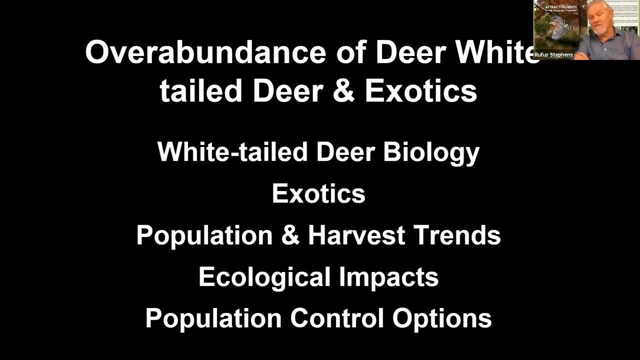 I mean, that's a great question and an interesting flip side to that is: do we? do we In other states? they will harvest as as much as we do in Texas Within a much shorter period of time, and wildlife managers have known for a long time that when you increase the length of the season, you do not typically increase the 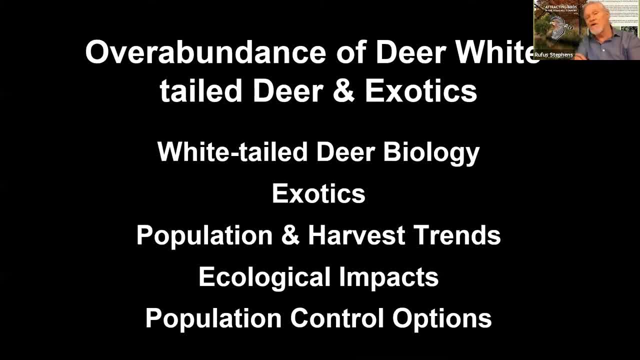 The take of the animals, People go- Oh well, I'll go hunting later. But the sense of urgency, when you only have a week or two weeks to hunt, you actually increase the harvest. So people are more focused on it and go out and they harvest more. 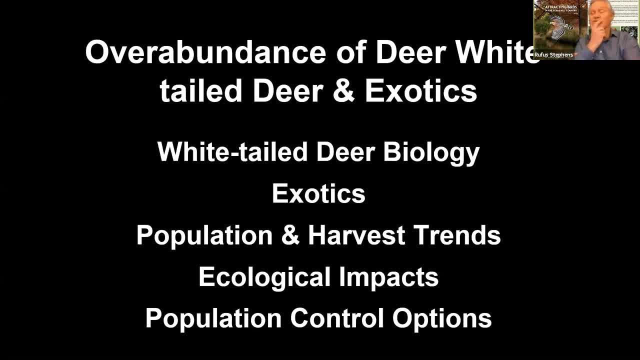 At at that time. So it's an interesting dilemma. So if so, even for quail. So if you wanted to to reduce the quail harvest, you could change the bag limit or you could lengthen the season, and you often will have the same result of. 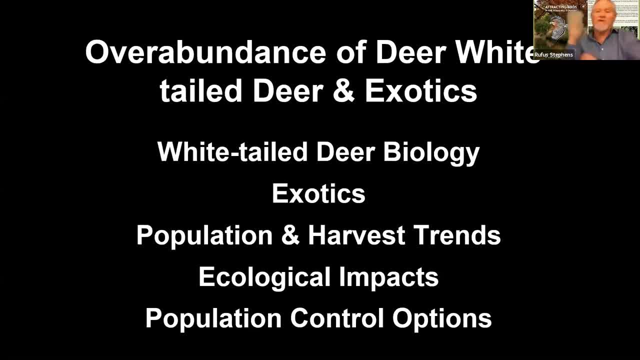 Decreasing harvest by increasing the season, because people will go- Oh, I'll go later, And then they don't go, But um, so that's an interesting aspect there. So Lucy would like to know: is there a study being done now of the storm and of deer dying? 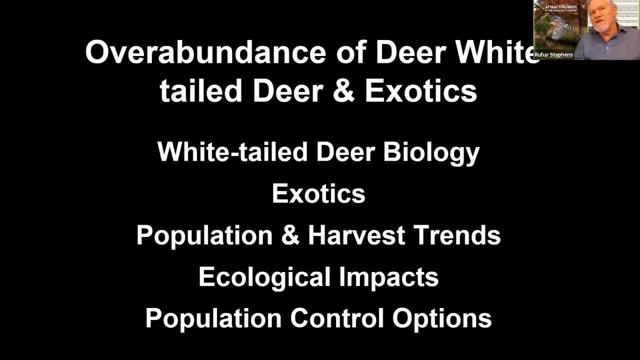 Yeah, no, there's, I'm sure there's nothing that it would be completely anecdotal. based on what? what they would they what where they would see? it is in their annual surveys which parks and wildlife does, Annual surveys across the state and the hill countries, divided up into several deer management units, and they, they sample the population based on those deer management units, not done by county, is done by groups of counties, And so I think I threw up a graph of RMU or DMU. 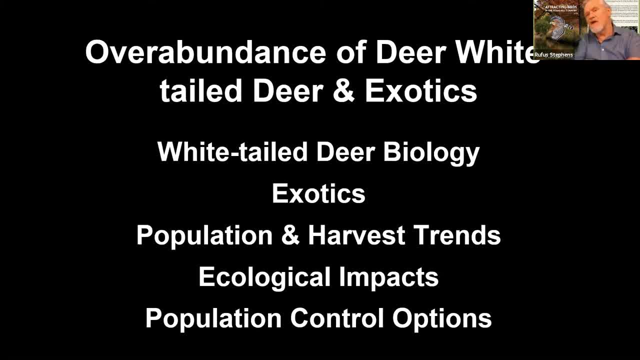 Deer management unit five which is around Kerrville but goes into Galaspe and Kendall and Bandera And so But the kind of Balcones Escarpment on the edge of the hill country, that's a different management unit. It might show up there. The other thing would be- and I said it's anecdotal, it will be- that people will call about deer that have died and they will call parks and wildlife and they will say we found several deer that died. 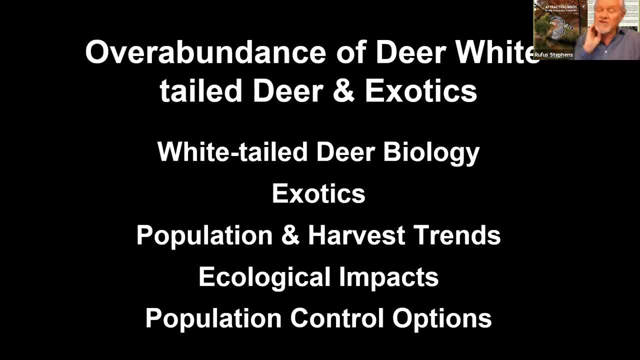 dive. usually the big thing when- just i remember this- that, while we're talking, is that what the worst kind of weather that we have for for, um, killing deer is, and especially axis, is a cold rain, and an axis cannot handle a cold rain, and so we will have large, relatively speaking large. 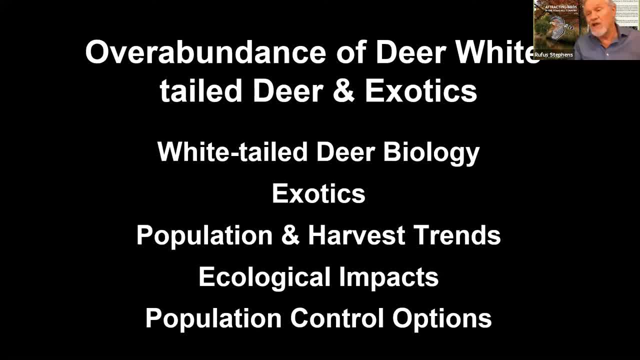 die-offs of axis in the spring when we have a very cold, cold rain. so, um, yeah, so. so we won't they. they will not be doing any surveys specifically of it. they'll know from people calling and then they may see it in and if it's significant they'll see it in their deer data. 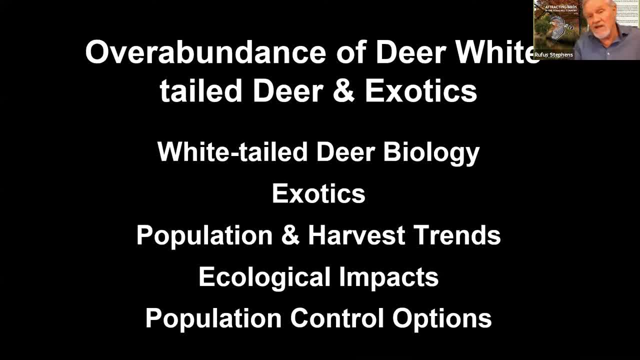 um, from from this summer, when they get that. so jeff would like to know how? how does hog populations affect deer population? yeah, so hogs don't, hogs will. they're very opportunistic, and so what he's what he's getting at is that hogs will, uh, if they come across a fawn, they'll eat it and uh, uh, you know. 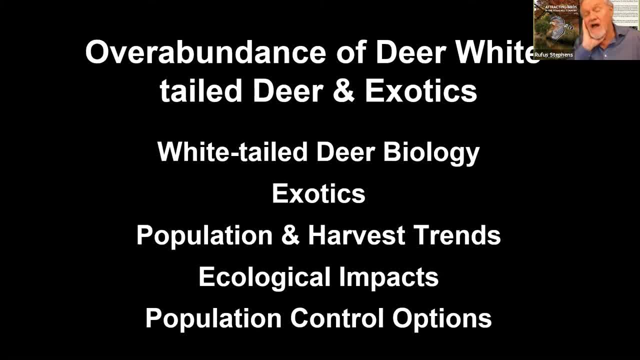 so they're. they're carnivores, you know they're. they're actually omnivores, so they'll eat anything they kind of come across. they'll eat plants, they, they, you know insects. they'll eat uh dead things they carry in. they'll eat uh uh live animals if they can, if they come across them, and it's easy. so 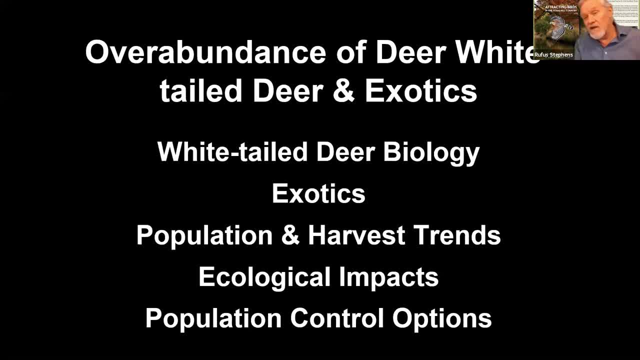 um, but their impact is not. i mean, we have pretty much ubiquitous hogs across the edwards plateau and it's not having an impact, a negative impact. are there fawns that are lost at? they probably are, um, is it? is it significant to the population? it's not, i don't know. maybe we may, uh, daryl, we may want to just do maybe one more, uh, you know. 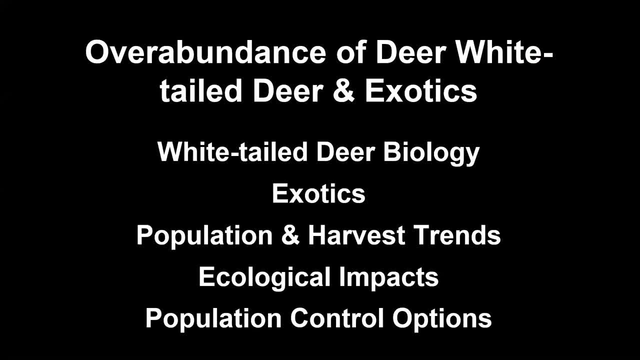 we have quite a few questions here, but i think we're running out of time, yeah. so, uh, if you want to ask one more, we'll do. we'll do that, okay. so, linda would like to know: how do you treat deer showing signs of parasites? uh, you do not use. uh, it is. it is illegal to uh treat with a uh. 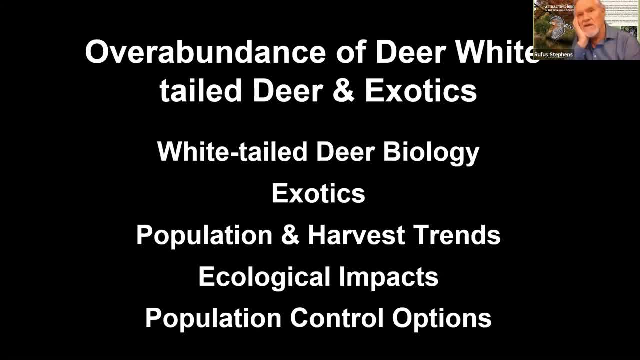 deer wild animals with a uh uh. so, for instance, of putting something out in their feed to try to control the parasites, that's that's illegal. the best thing to do is to stop feeding, because it's that concentration around the the feeders that's causing them to. 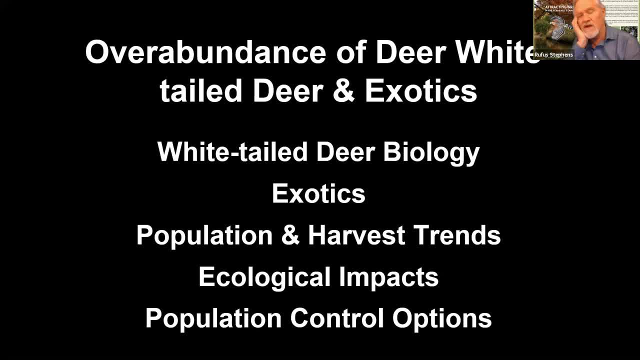 pick up high parasite loads. if they're able to move around through the landscape and feed on natural foods that are not parasites, they're not going to be able to control the parasites. they're not going to be able to control the parasites. they're not going to be able to control the. 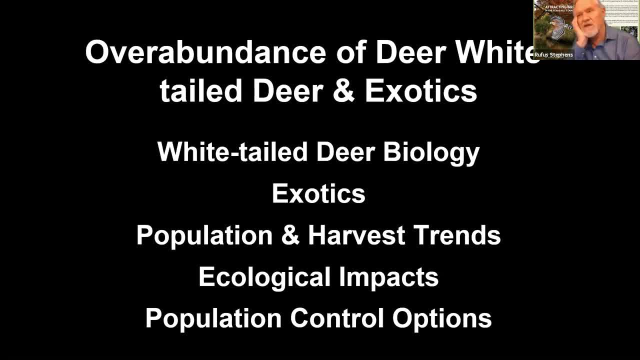 they will not pick up as many parasites, it's them being concentrated, so that's the best thing you can do for them and it's and it's not legal to to go out and and treat wild populations. so would not, would be happy, wouldn't be happy. so, uh, i i'm going to skip over this. this is just kind. 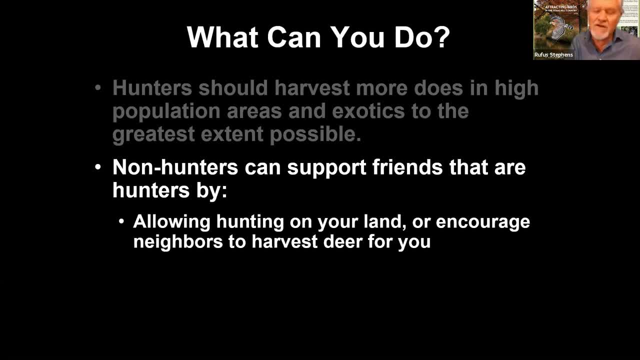 of what you can do. we've already talked about some of it. one of them is: you know harvest deer if you want, if you can, and i'm going to skip over this. this is just kind of what you can do and uh that, uh. also, if you're not interested in harvesting, you know work with friends. 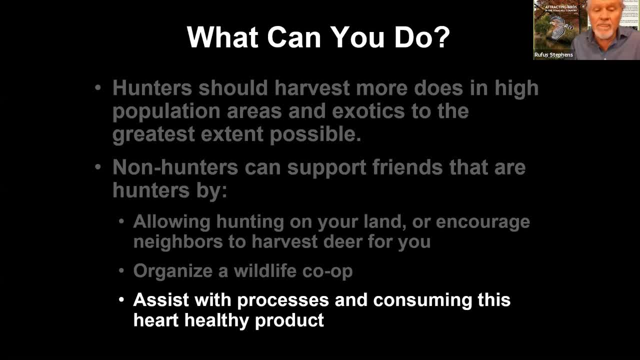 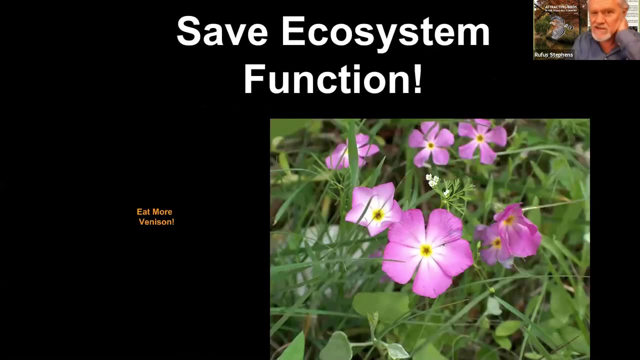 do a wildlife co-op, um, and assist in processing and consuming this heart healthy product. actually, i'm a heart patient and it's very low uh food. the other thing you can do is grow priority plants, the ones that they like, and cage them where necessary. so the best thing you know for to save our 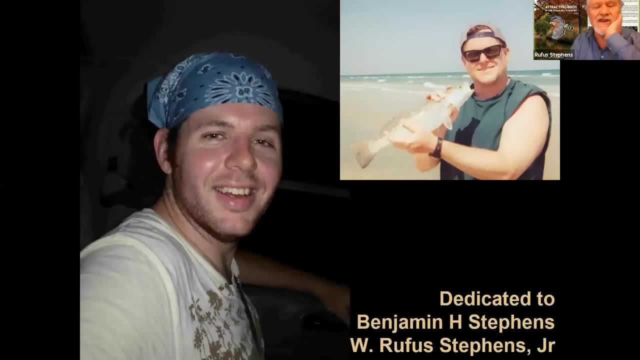 ecosystem function is to eat more of them, so i'm going to skip over this. this is just kind of what i'm going to skip over this. this is just kind of what venison, uh, the um, i i do. i dedicate my presentation to my brother ben, and to my son ruth, um, and so. 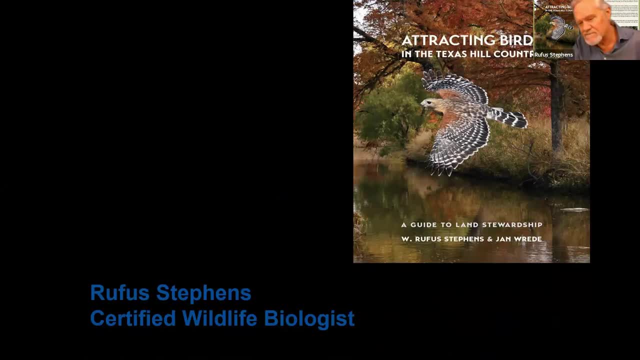 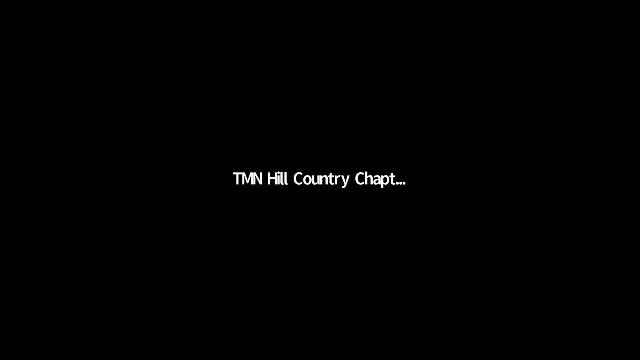 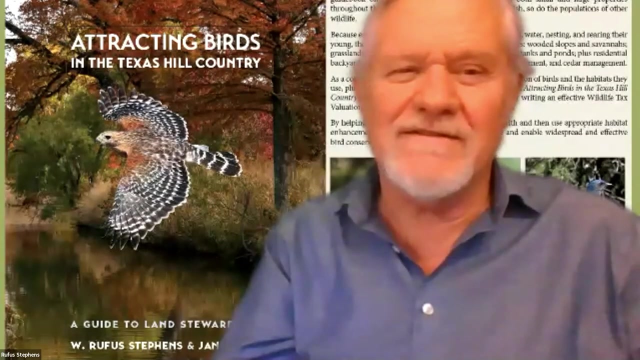 with that. thank thank y'all very much for having me. well, that i i got a lot of. that was a very interesting presentation, so i do appreciate it my pleasure. yes, we, thank you very much. you bet it was my pleasure. it is probably one of the the toughest, um, you know, uh, management issues that we have, and i think 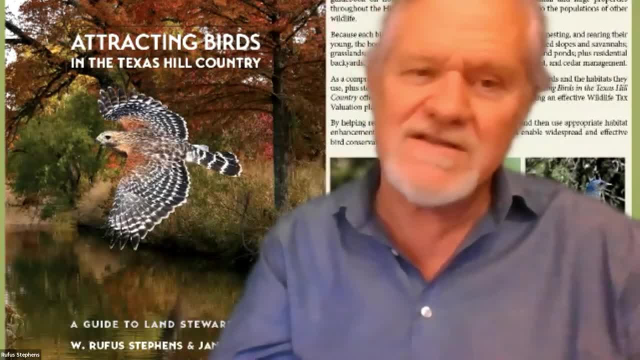 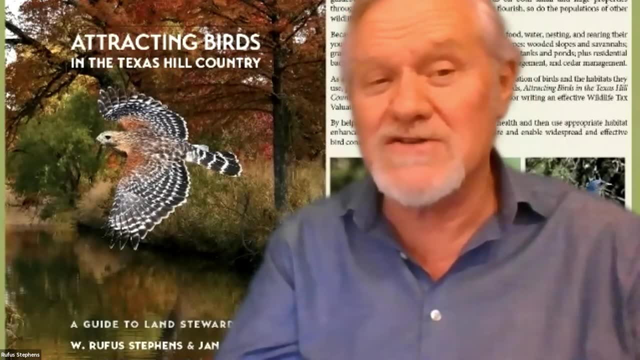 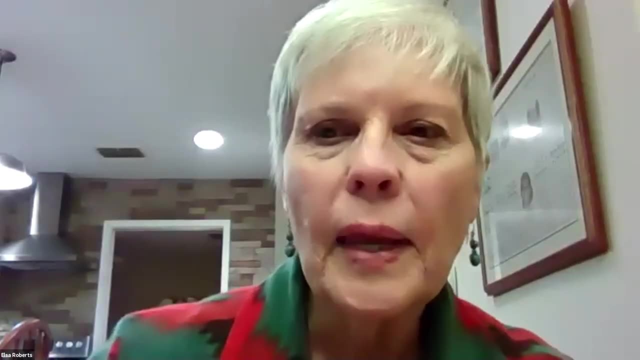 everybody's got an opinion and and uh, and it's difficult, it's not an easy problem to try to solve, and so, uh it it. it deserves good discussion and and probably a lot more in the future. so, but, thanks for having me, thank you. thank you earlier today with with the class, that was great.